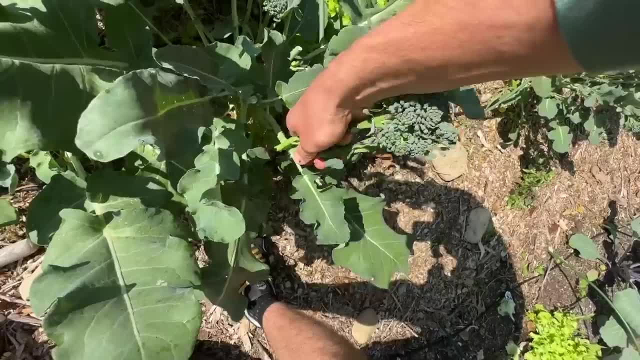 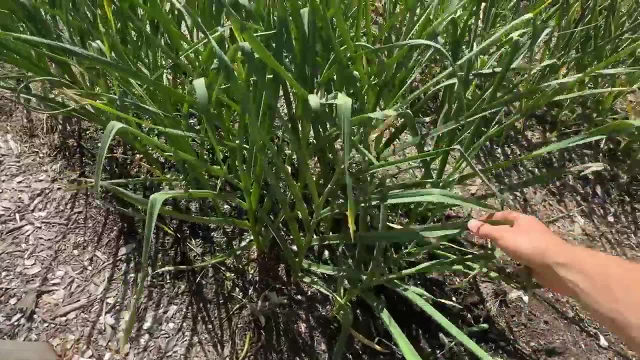 it off and it keeps creating these little shoots. So the harvests come early, but they also just keep coming for weeks as you just break them off Over here. I've showed you this a few times. This is my garlic patch and we're about a month. 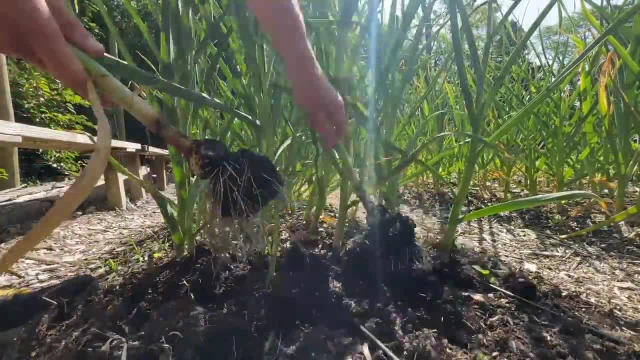 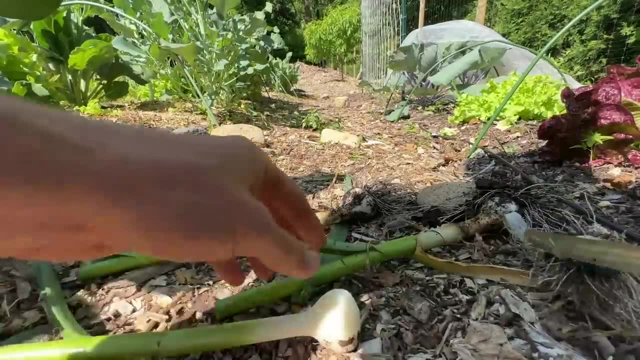 a month and a half from really doing like a proper garlic harvest, but I just continue to harvest this spring, or what they call green garlic, which is just young garlic. You can see, here the heads are really starting to develop. You can see, here the heads are really starting to develop. You can. 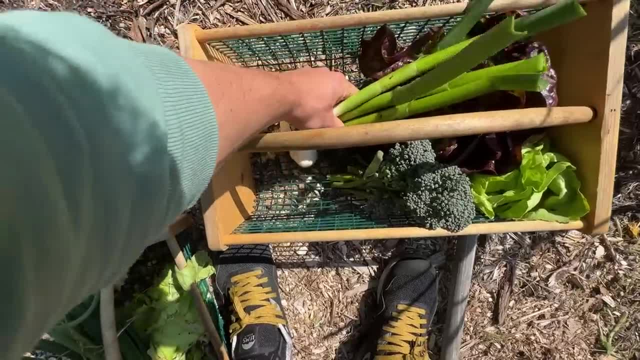 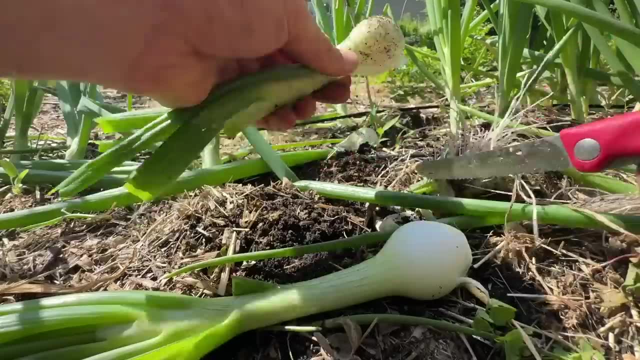 see here the heads are really starting to develop as it gets warmer, So I can now use this just like a normal head of garlic. Over here I have a bunch of onions growing, just like the garlic. As it gets warmer the heads are starting to get bigger. but I've just been harvesting these spring onions. 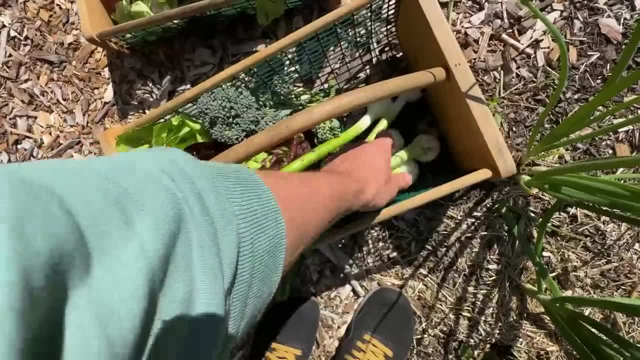 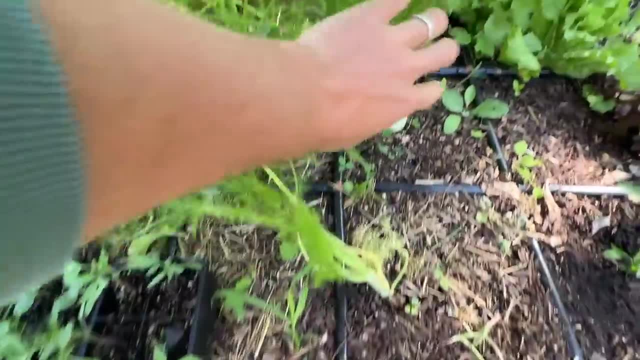 which are great, as I need them throughout the season. We'll head over to the raised beds now for just two more things. First, in this cold frame, I've got a few things grown in here, but I'm after this big ass fennel, which is my favorite aromatic to use. We're going to cook. 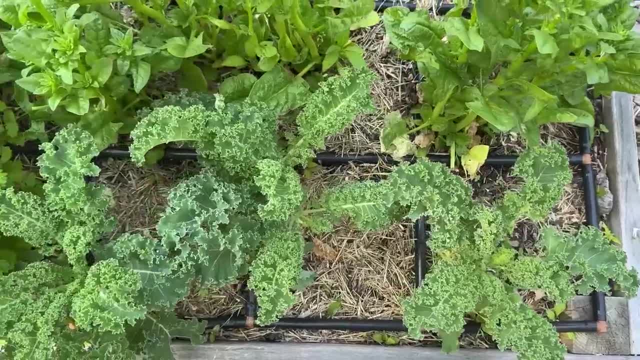 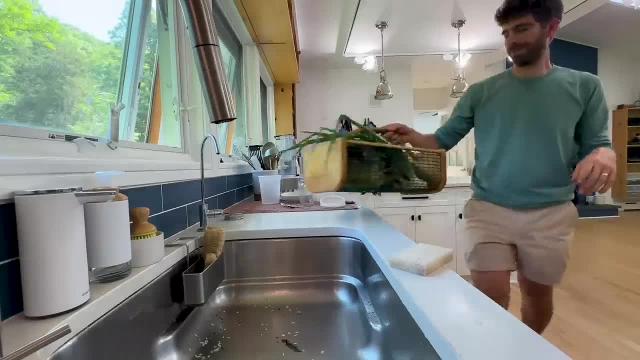 that up in a pasta. And then finally, over here I have a bunch of garlic that I'm going to put in. here I have some beautiful kale, So I'll just collect a little bouquet of that And I'll head inside. I'll process all of this, meaning clean off all the bugs and dirt and we'll get into. 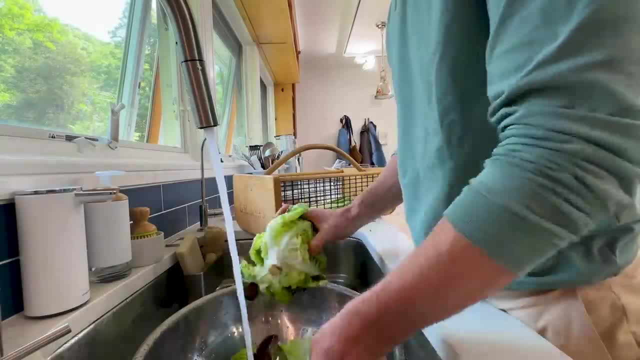 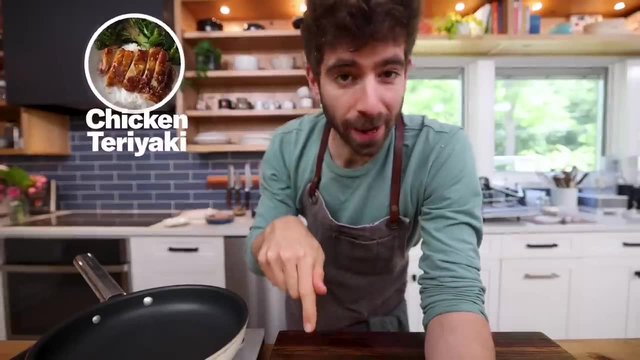 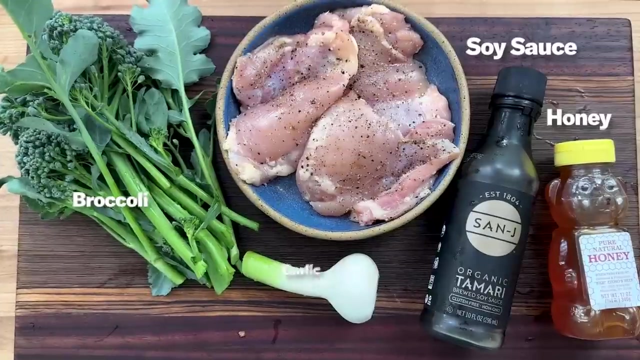 these recipes. Now, one of my most popular recipes of all time on the channel is chicken teriyaki, which makes sense because chicken teriyaki is the best. Now, what I am about to show you is a simplified five ingredient version of that that is still incredibly delicious, but comes together. 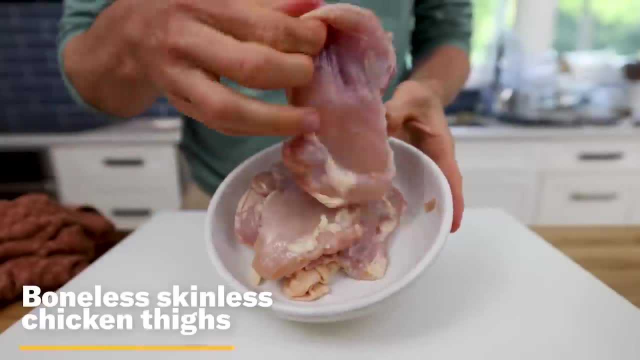 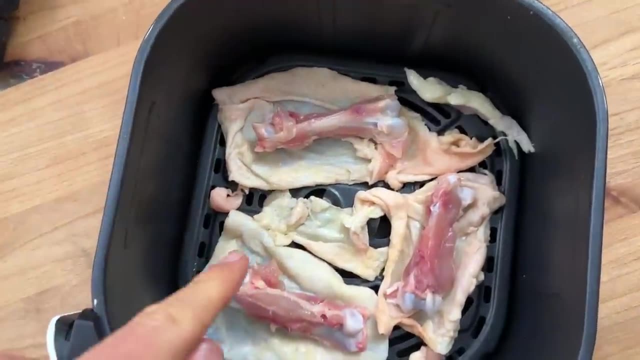 much faster. So right here I have some boneless, skinless chicken thighs- and these were actually bone-in skin on which I took off both of those things and placed them in the air fryer and air fried them for 15 minutes on 350 degrees Fahrenheit, And now we have this crispy chicken. 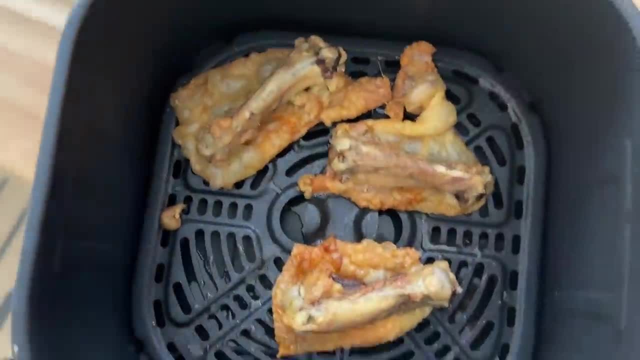 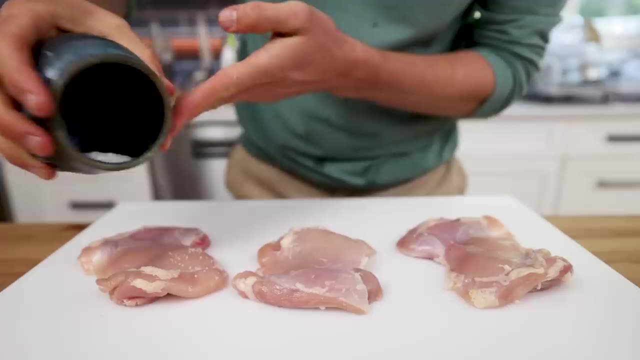 skin, which I like having as a separate entity in this dish, because we're going to cook the actual chicken in sauce, which would make the skin soggy, So we can actually garnish with this later on. And for the chicken thighs, I'm just going to season them with salt and pepper on the 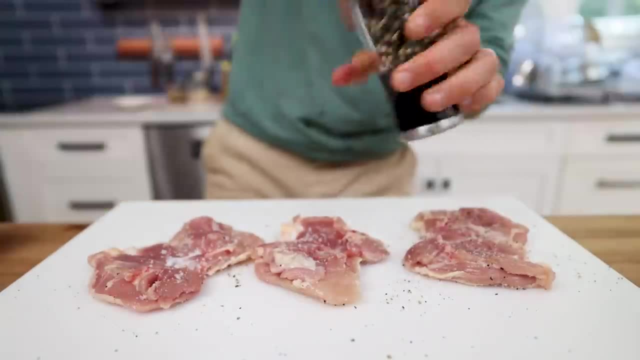 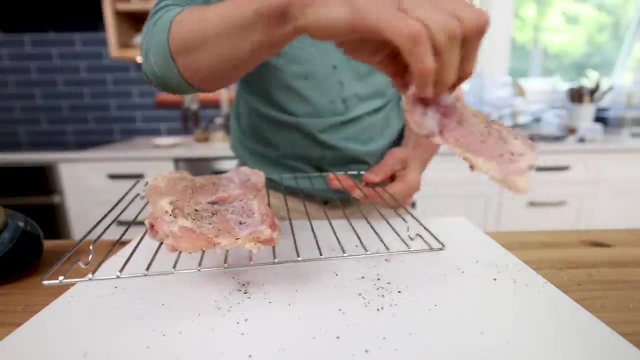 both sides And you can go a little bit lighter on the salt, because this dish does have a good bit of soy sauce in it. And if you do plan this ahead of time, throwing these in the fridge for like 12 or even 24 hours max is going to give you an incredible final product. But even if you just 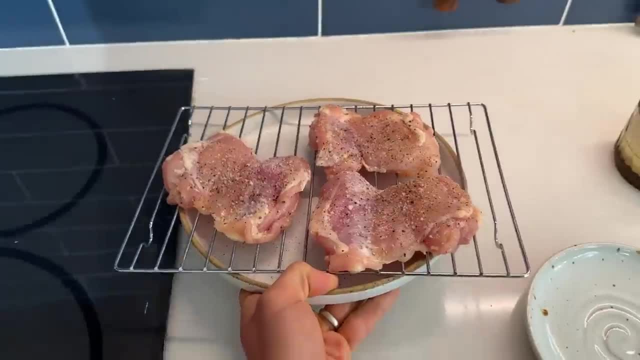 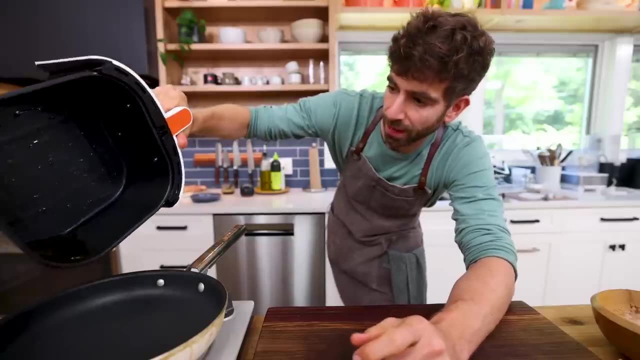 have 15, 30 minutes. just let them sit out at room temperature and let that salt do a little bit of work. Here is the rendered fat that came off that chicken skin. I will just dump that right in to this preheated pan. So we're cooking this chicken in its own. 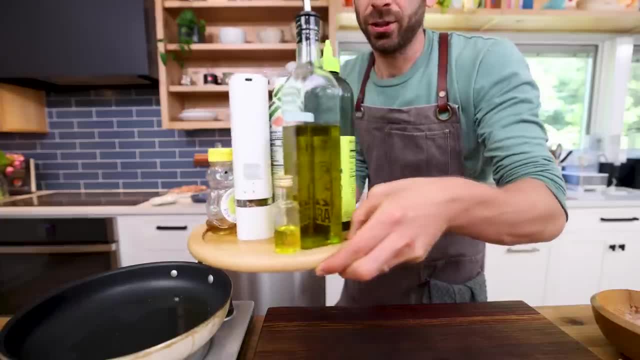 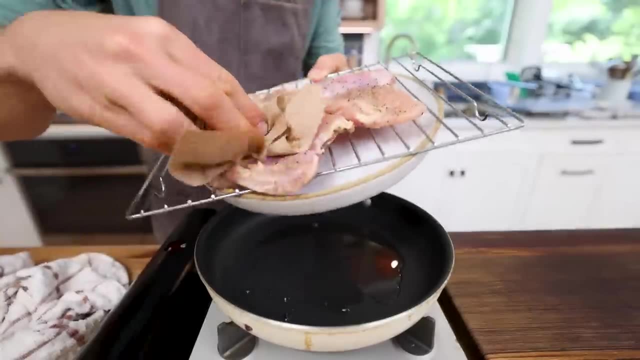 And I'm going to take a little bit of the rendered fat, which is ideal, But, of course, if you don't have the rendered fat, just use any of your standard oils. So these have been sitting out for just 30 minutes. There's a little bit of moisture that's being pulled from the salt, So I 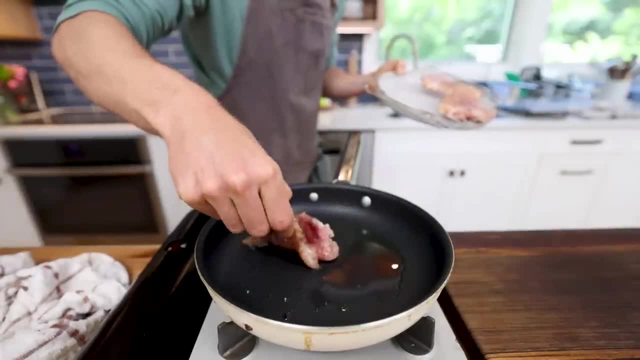 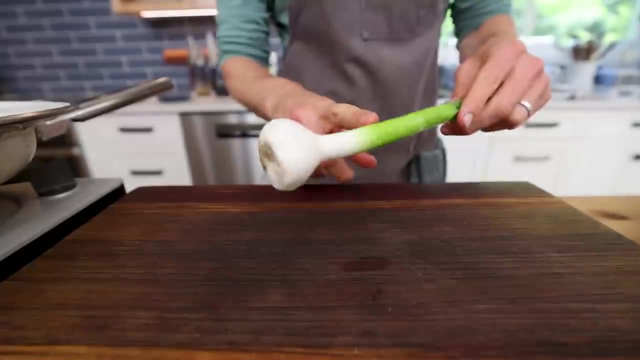 will just pat that off and we will get these frying up in the pan. Turn that up a little bit, Two, three, And I'll just get the splatter guard on that. And really the last main prep for this dish is chopping garlic. And if you've never seen young spring garlic, pretty cool, It looks like. 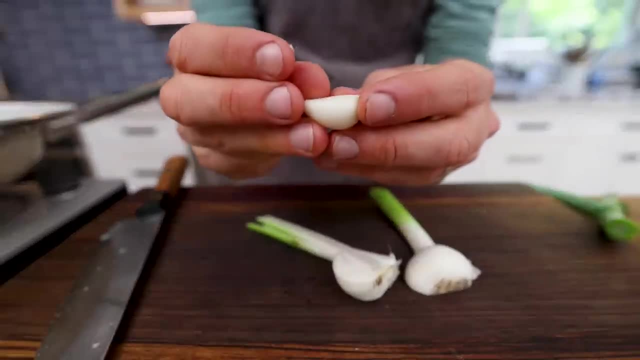 it's been chopped up in a few minutes, but you can still- Whoa, oops, You can pop out these individual cloves, which I'm going to do now. Look at that, That's so neat And I'll just give. 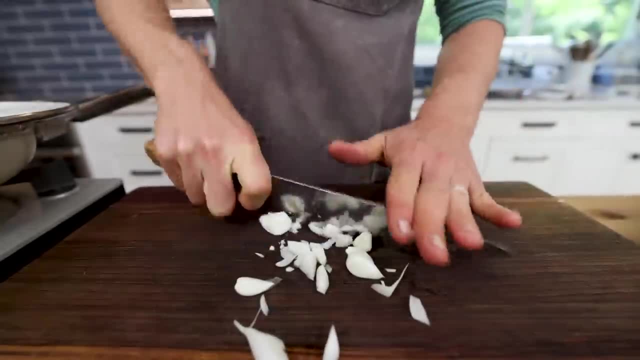 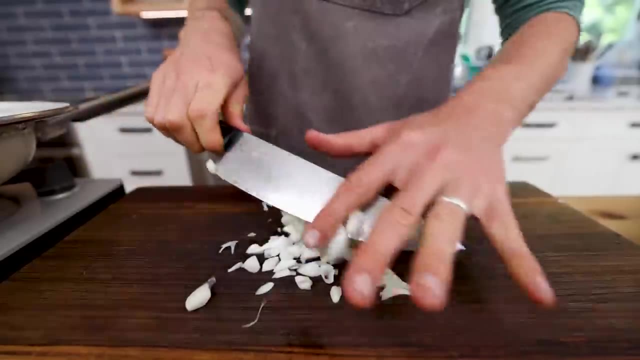 this a rough chop, And most of you, of course, are going to be using regular garlic. The only difference with this is the younger garlic is a little more subtle. The flavor hasn't intensified yet, So I'm going to use an entire bulb here, Whereas for you a few cloves of. 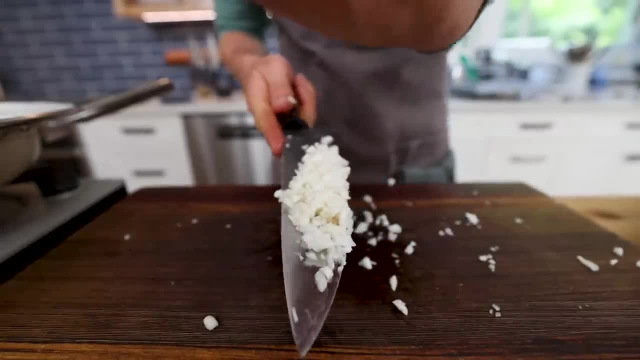 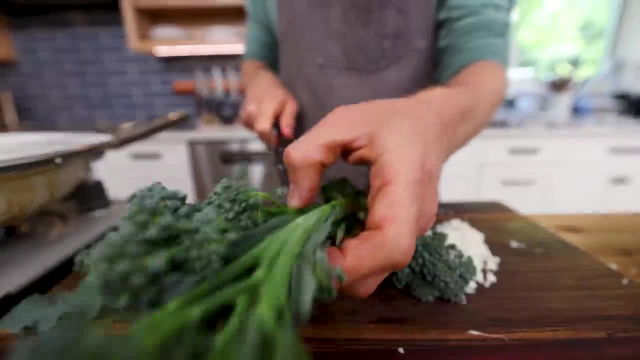 garlic will get the job done. Boom, It can be pretty rough like that. Now for the broccoli. depending on what type of garlic you're using, you can use a few cloves of garlic, but if you're wondering what type of broccoli you're using, the goal is just manageable size pieces, So just. 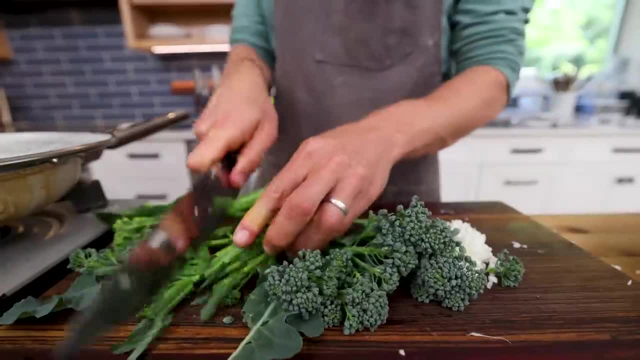 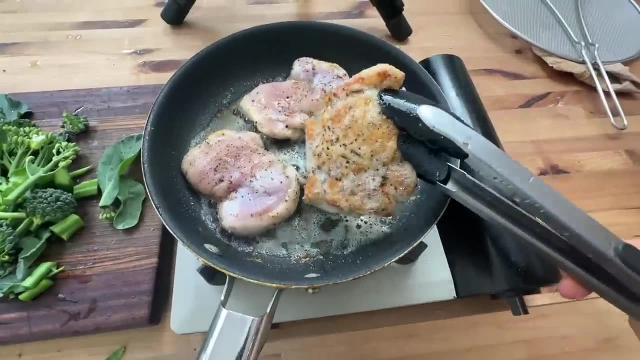 cutting off these tops. I can give them a rip and then chopping some of these stems down a little bit, And that should do the job. Let's check in on this chicken. Where are we at? Oh, not bad, Needs about another minute And we can undercook it slightly because again it's going to cook in. 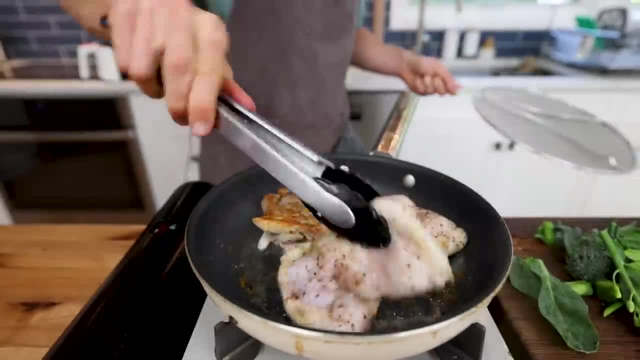 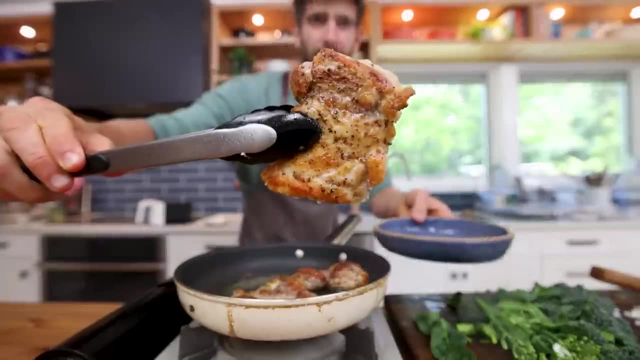 the sauce later on. All right, Let's see. Okay, Perfect, I'll just cook this for about two minutes on this side. All right, Chicken Coming off Just onto a little plate here, Looking good. Now we've got a lot of residual. 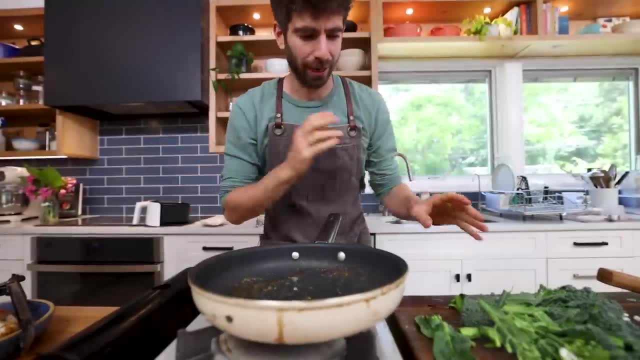 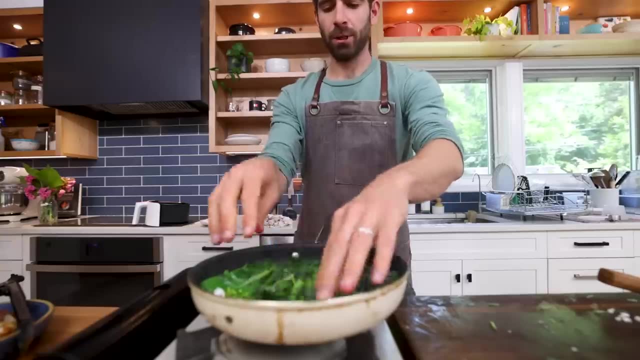 goodness in there. Never. you know this by now. never get rid of that. We're going right in to that. Whoa Excess water on that broccoli- And what I love about this sprouting broccoli: you can just kind of stir fry it pretty quickly And we'll just cook this for maybe a minute. 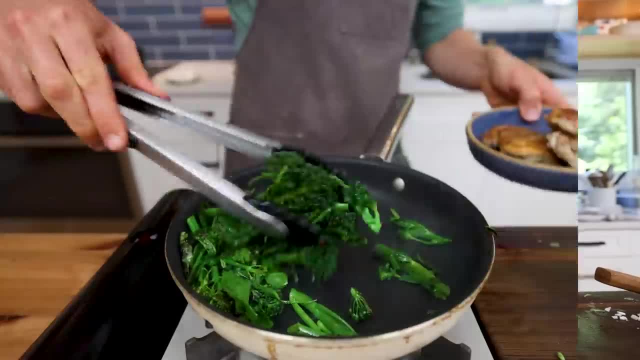 two minutes until it has some nice color. All right, So that's done. Nice and crispy, We'll pop that right on to the chicken. All right, So that's done, Nice and crispy, We'll pop that right on to the chicken. All right, So that's done, Nice and crispy, We'll pop that right on to the chicken. 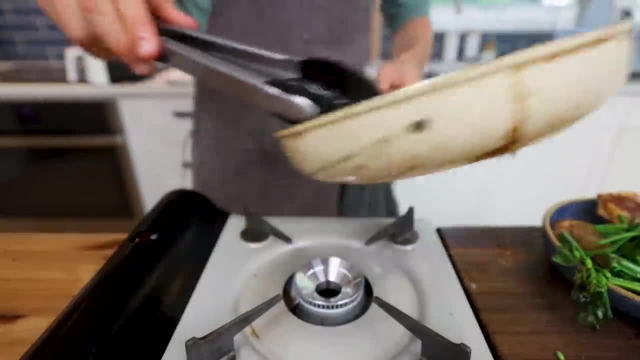 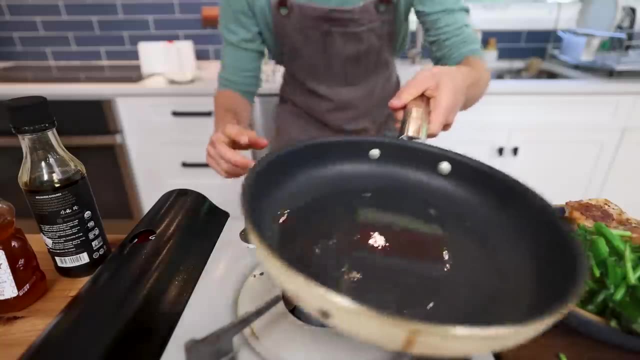 And we'll turn things down a lot. We don't want to burn any garlic. I think I've got a little bit more of this fat, Just a little bit. Is that enough? We'll add a little additional. All right, Now, this happens very fast, So be prepared with your ingredients, which is just soy sauce honey. 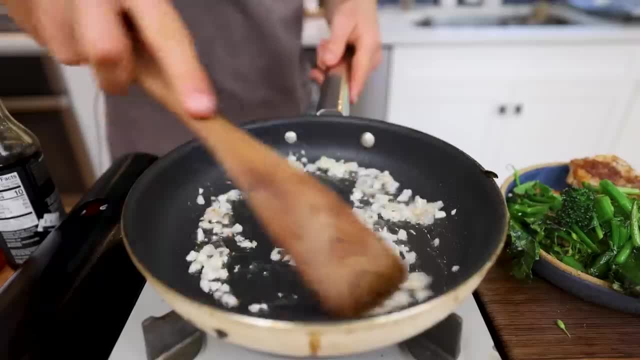 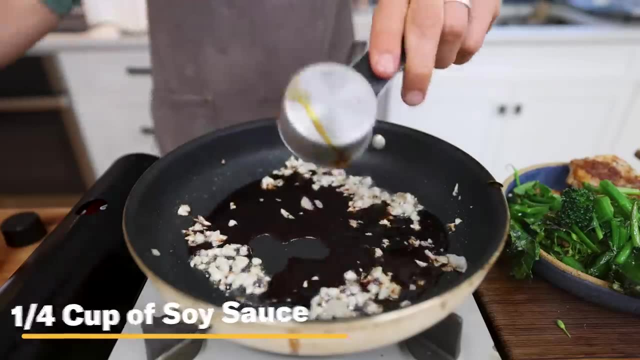 and garlic. Just keep moving that garlic around until it's nice and fragrant and a little bit soft, And then I'm going to go in with a quarter cup of soy and just under a quarter cup of honey. This is your sweet and your glaziness. 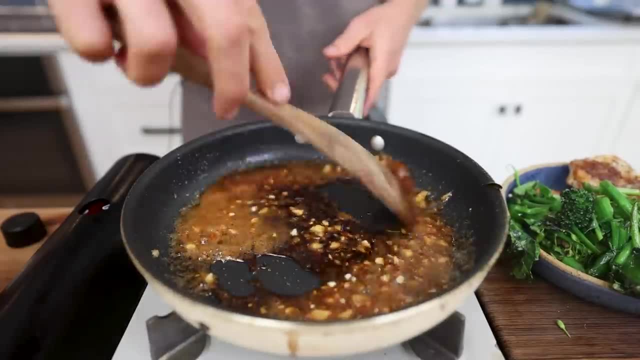 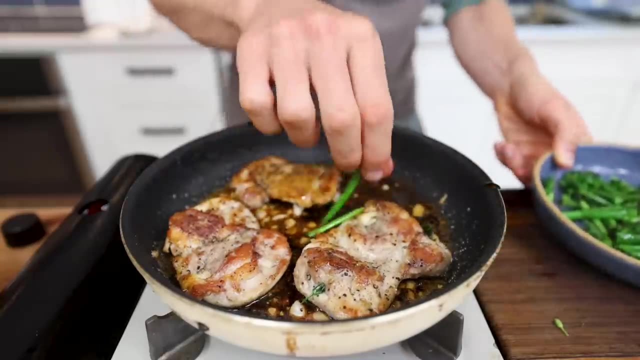 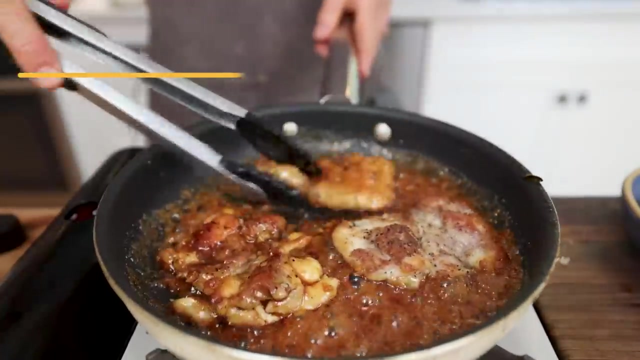 And just give that a stir And since these are a little undercooked, I'm going to throw in my chicken thighs along with any juices that came out. the chicken And on a medium heat we'll just let that reduce and get nice and sticky To plate this up. really simple Got. 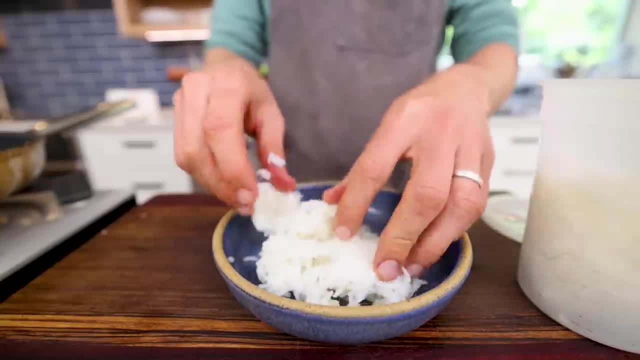 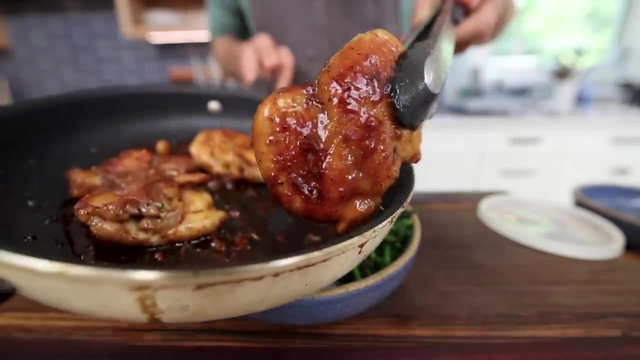 some leftover rice I just threw in the microwave. Just get a little bit of that on the plate, Got some broccoli in there And then look at these glazed up soy garlic chicken thighs, And then, of course, look at this sauce. 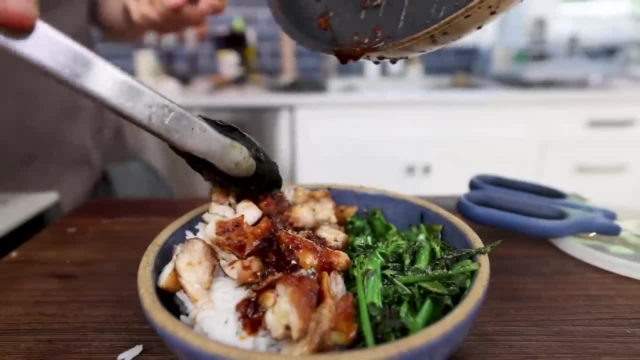 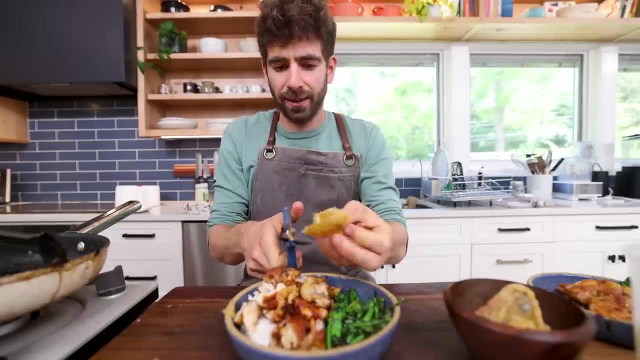 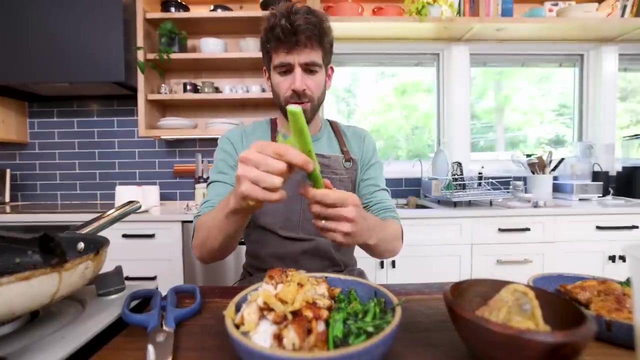 Garlic, soy honey. It's all you need. Oh my God, I almost forgot Crispy skin. Again, the isolation here. So you preserve that skin When you're working with only a few ingredients. you got to get crafty. Actually, speaking of crafty, this is a bit of a cheat code You can. 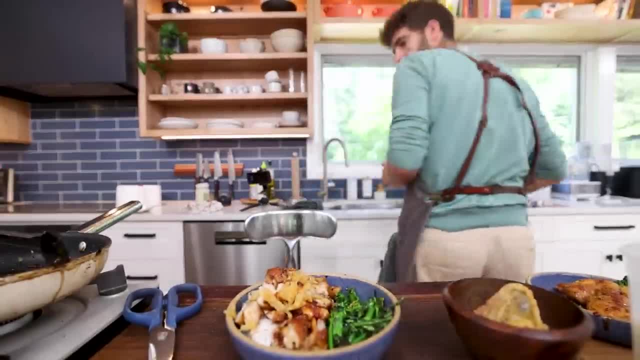 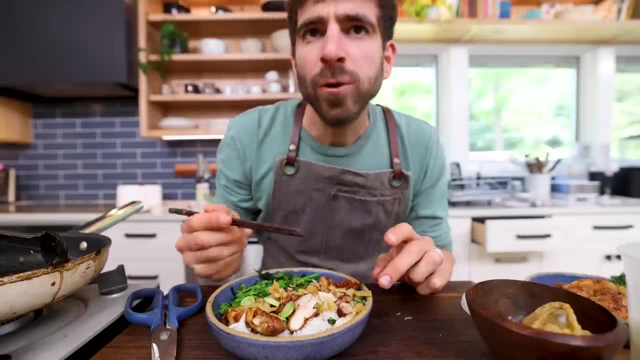 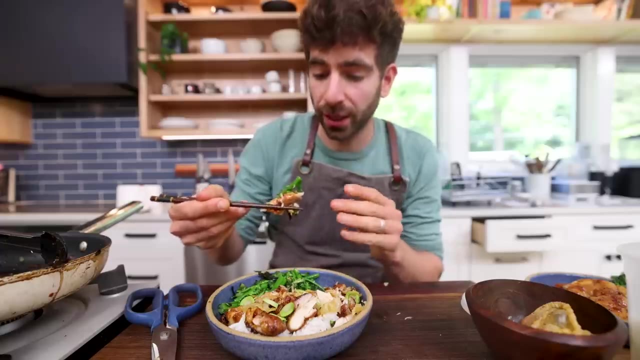 use the garlic ends as scallions, pretty much. So I'm just taking that And then I'm just going to bring this dish to the next level. A few of those Now we're talking. Look at that, Oh my God, Salty, sweet, Definitely reminder under-season that chicken, That sauce is packed. 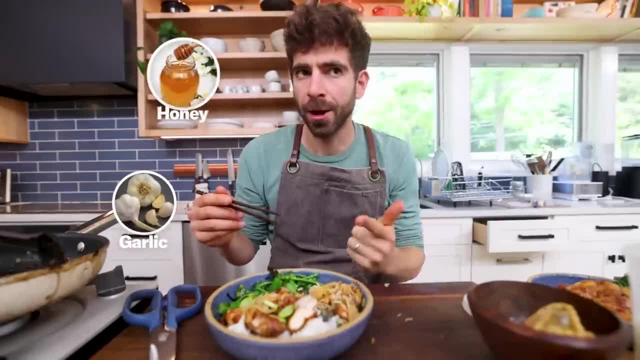 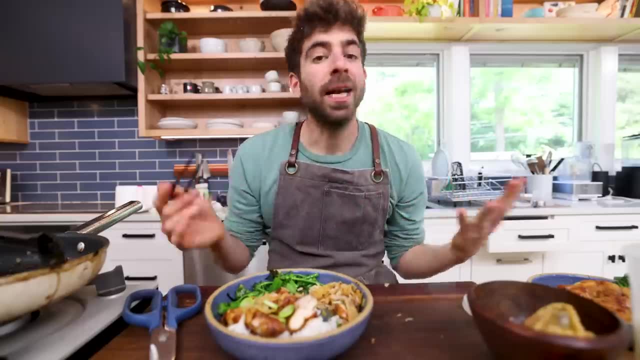 in a salty punch. Most of you, I'm guessing, will have garlic, honey and soy sauce in their pantry at all times, So this is a perfect dish to rely on if you don't have extensive ingredients to really build out a fancy sauce. So before I get into the next recipe, I'm going to give you a. 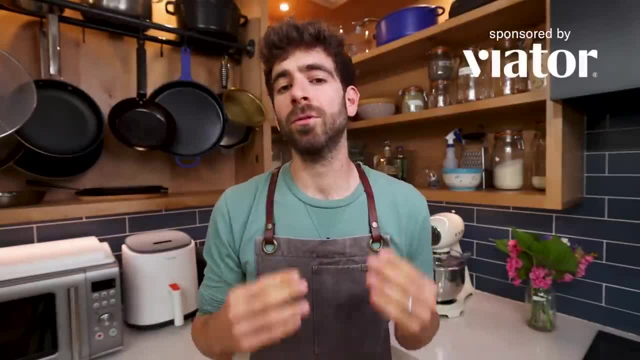 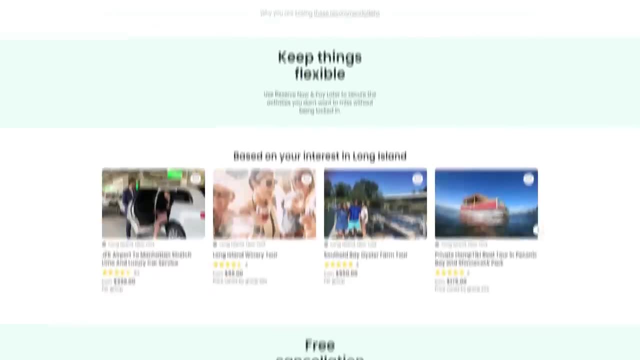 recipe. I want to tell you about today's sponsor, which is Viator, And, with over 300,000 travel experiences, it's the premier place on the internet to book your next epic experience. And what I love about Viator is that, at its core, it's just a great search engine for finding a new 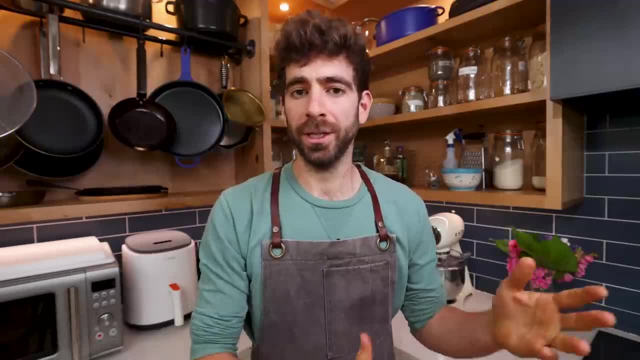 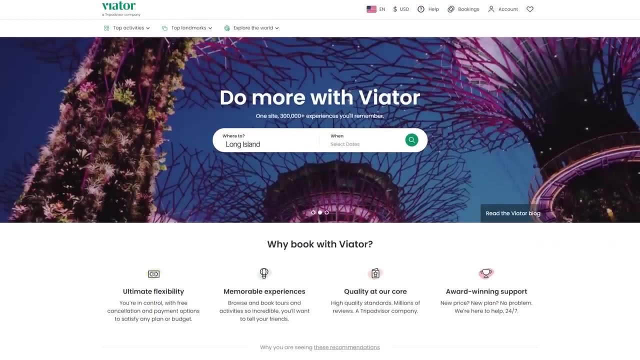 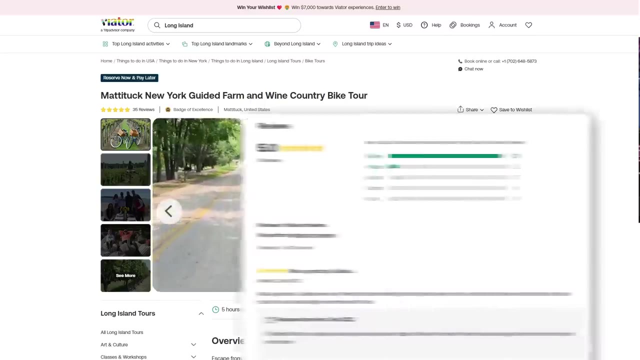 experience. So for me. I've got two little kids and I wanted to book something fun with my wife, but it needed to be close, It needed to be somewhat local. So when I was searching for a weekend farm bike tour which is right up my alley and with Viator's detailed descriptions- 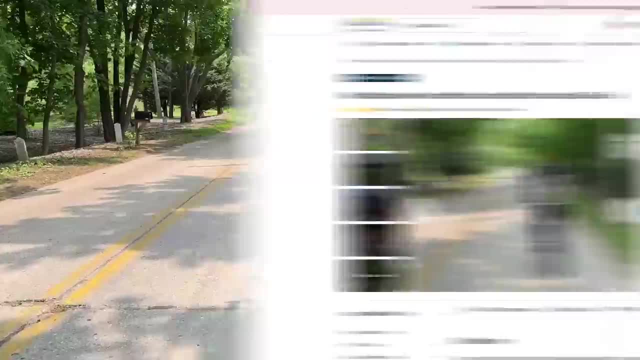 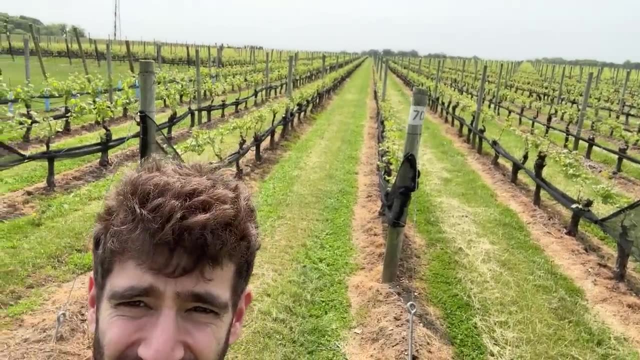 and real travel reviews. it was kind of a no-brainer to book this bike tour And this excursion totally blew me away. The North Fork is just a hub for agricultural tourism. We visited a few vineyards, a bunch of farm stands and sampled some great local food and really just got to take. 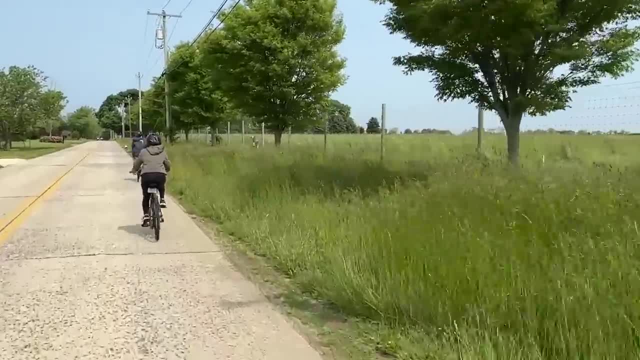 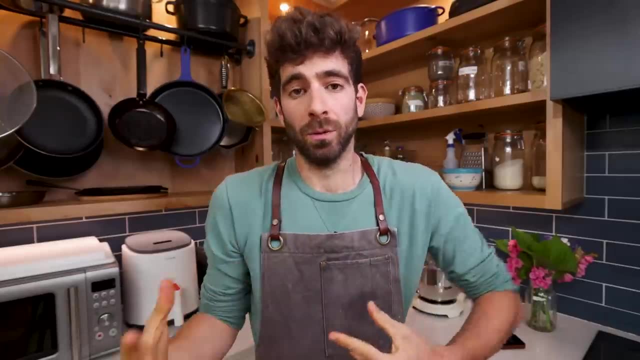 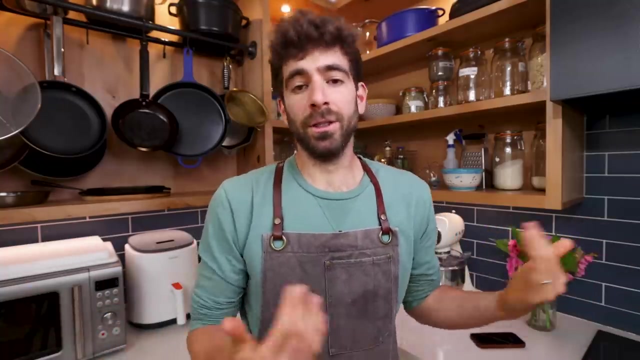 in some amazing scenery via a nice calm bike ride around the North Fork, And booking is an absolute success, which is great when you are trying something new. So maybe you've got a trip coming up sometime soon and you're looking to build out your itinerary, or you're like me and you're just 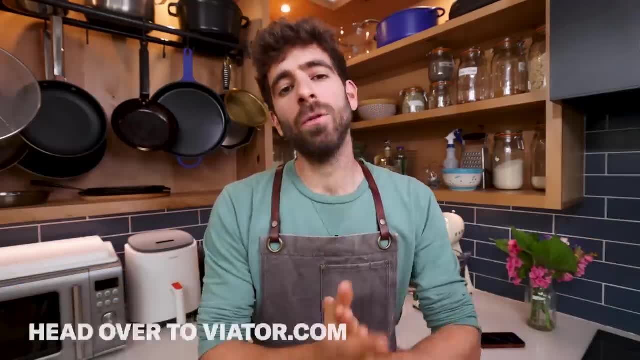 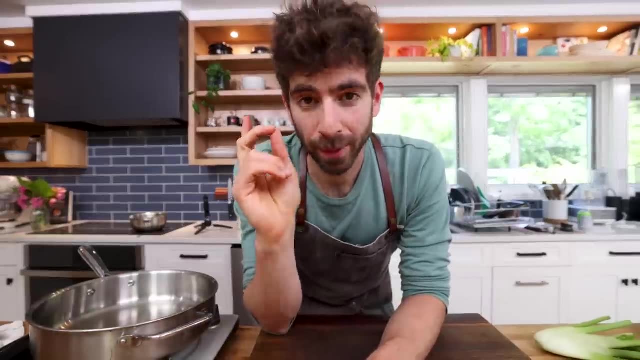 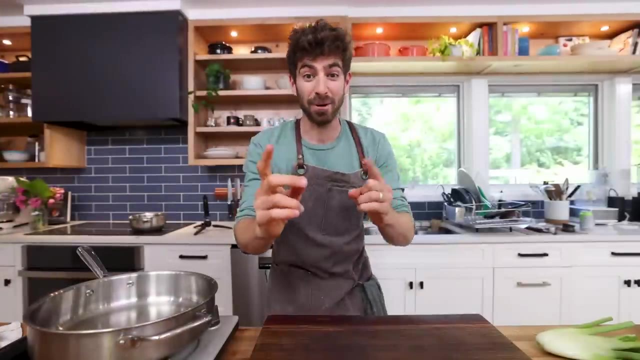 looking to do something locally. that's fun. Whatever it is, head over to Viatorcom to book your next travel experience. You will not regret it. So up next, I am making pasta, because pasta is simple, which is why it is the best weeknight dinner, And this one is inspired by a very special 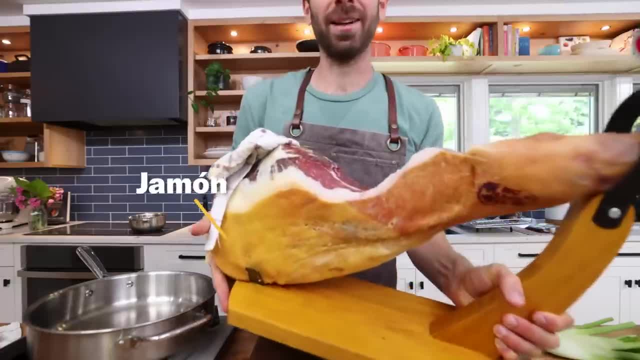 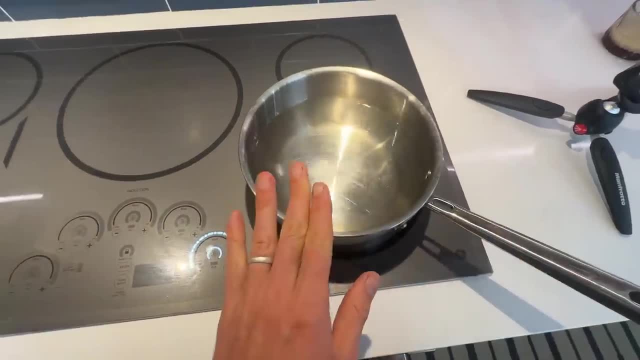 guest: Ha ha, The jamon. Oh, look at this thing. I've kind of made a dent, But before I carve this up, I will just preheat some water for blanching the kale and boiling the pasta, And then I'll get this pan. 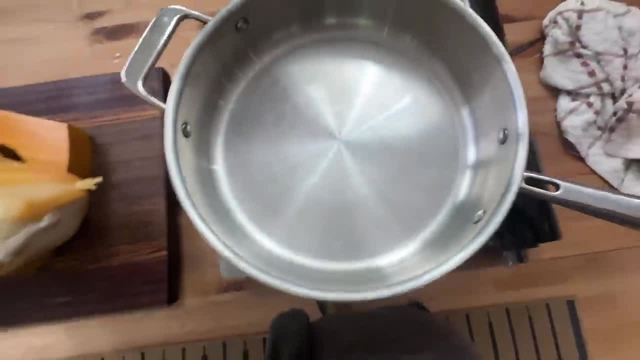 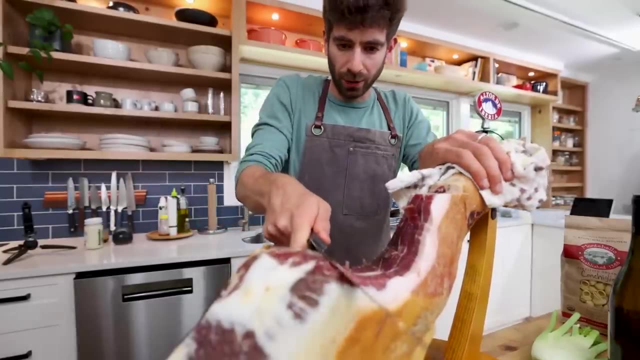 right here, which is a nice wide saute pan with a high lip, my favorite for making pasta. I'll let this heat up on a medium heat. So, as you can see by the looks of it, I am no jamon carving expert. 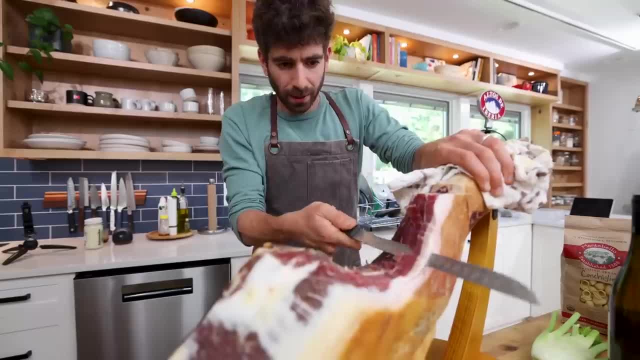 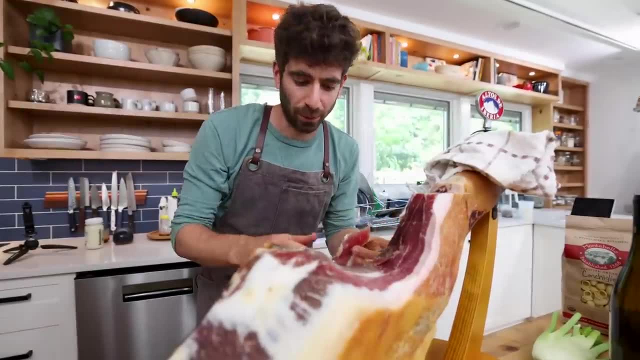 but honestly it doesn't matter that much. Any thickness is gonna be good. Some nice fat to ratio, And this was. It was $199 on Amazon, one of the cheapest ones you can get. It's pretty damn good, I will say. 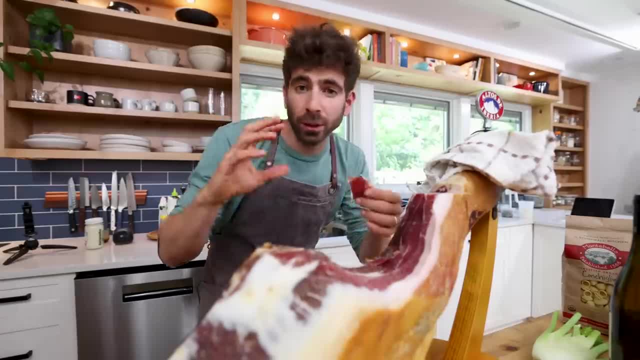 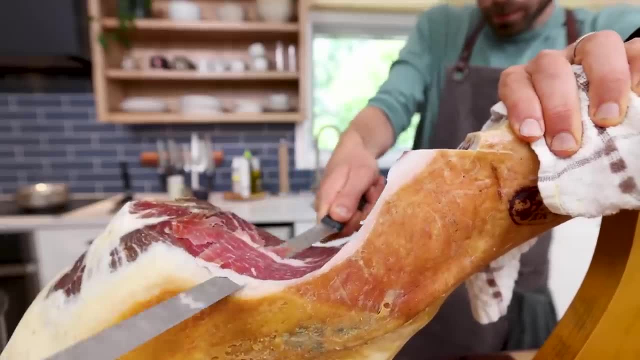 and it is lasting me a while- Like a great investment versus spending $20 on a little packet of prosciutto from the market. It's really been fun to have. I'm just gonna keep slicing this up into little chunks and I'll get it frying off, So it's pretty thin there. That's almost see-through. 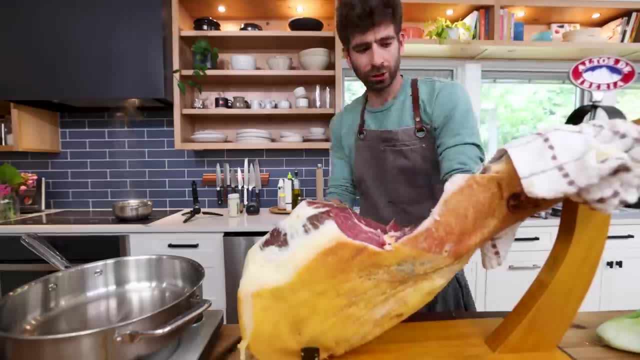 jamon. All right, one more piece, That should do it, And we'll take the jamon out of steam. Ha ha, Now the pan is preheated. I'm just gonna do a tiny bit of this. I'm just gonna do a tiny bit of this. 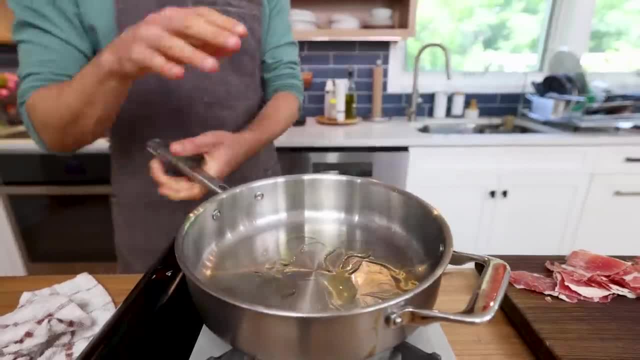 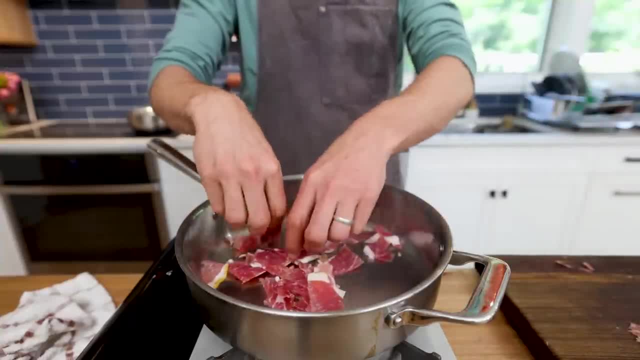 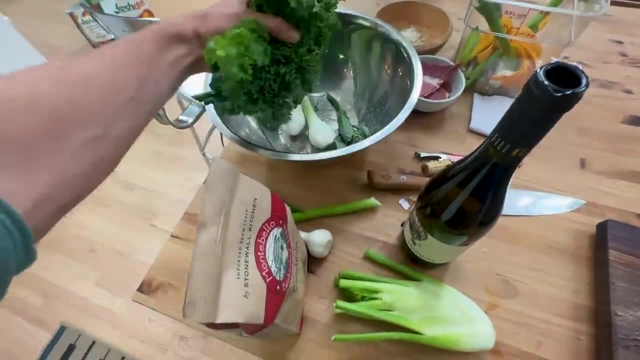 started. And, of course, you can use pancetta, you can use prosciutto- Any cured meat with a decent bit of fat is gonna give you a lot of flavor. Now, while that is rendering, I'm just gonna take this handful of kale, pop it right into here to blanch, which will only take probably. 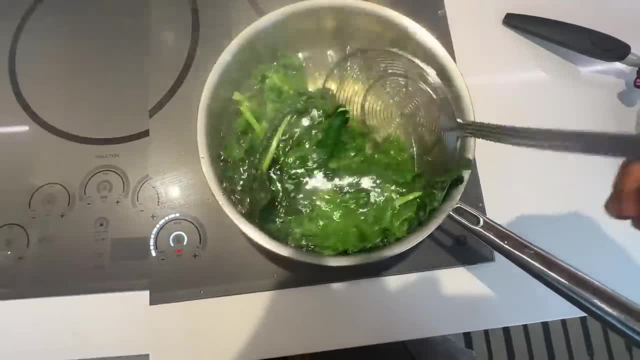 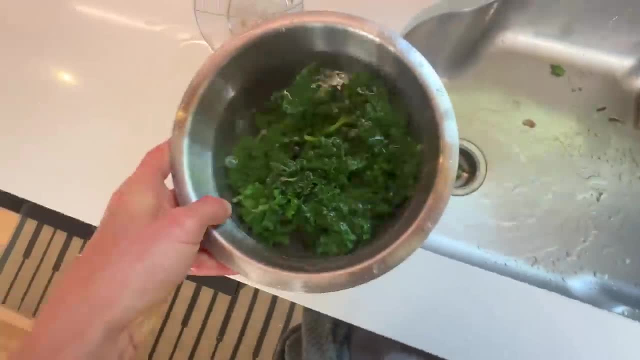 30 seconds to 45 seconds. You can see it goes bright green right away and then that's done. You want to preserve that freshness? Just get that in a bowl of cold water, Just let that sit and then, once this greenish water is back up to 10, I'm gonna go in with my 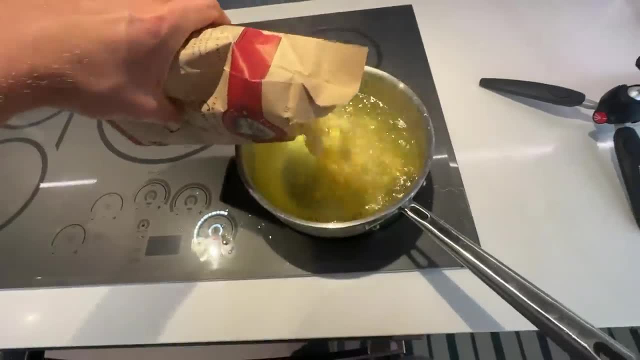 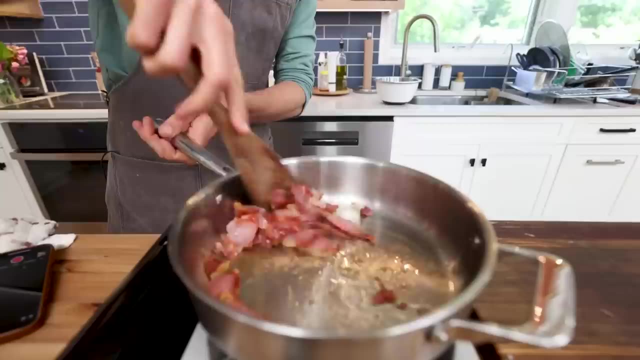 pasta, which are these bigger elbows? Says about nine minutes. I'm using about 12 to 16 ounces. Hit it with a little bit of salt and we're off to the races. We just want to keep moving that around so we get a nice even crisp and keep it on a nice low heat. We don't want to burn this ham. 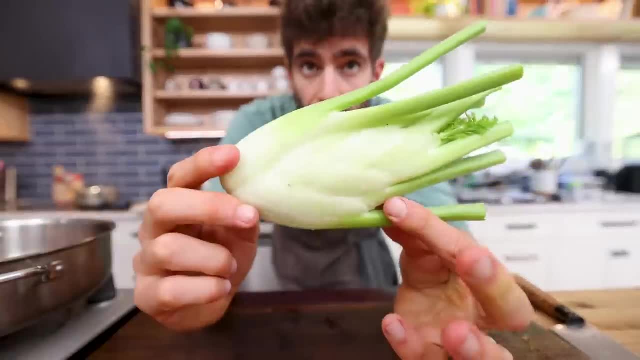 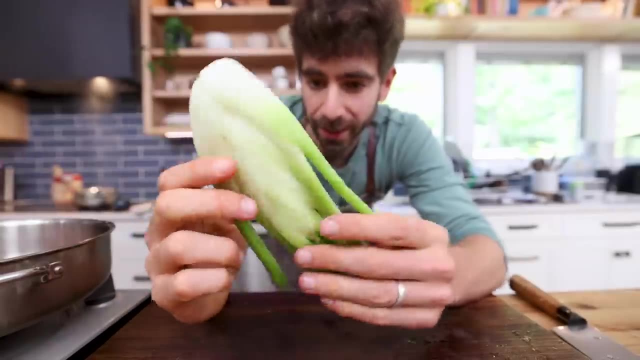 And the final prep is just cutting up this fennel. If you don't have fennel, if you don't like fennel, I would first say try just caramelizing it in some oil. You'll become a fan. But you could totally replace this. 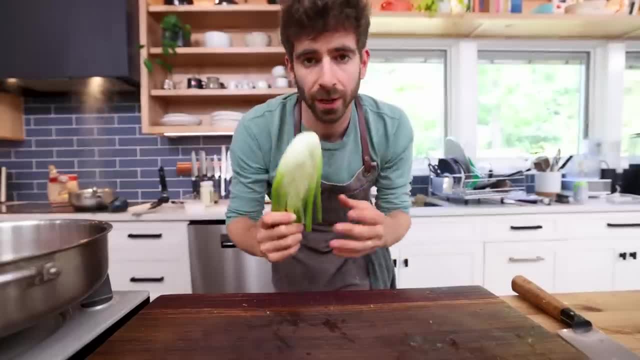 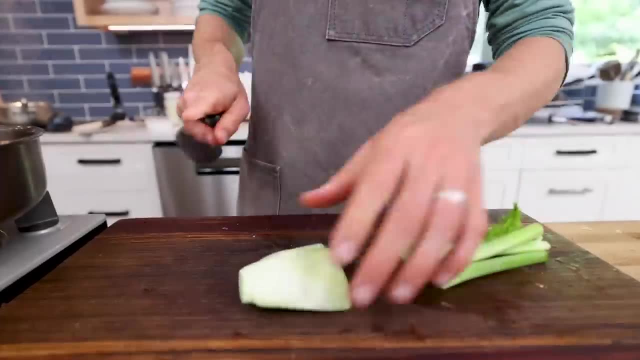 with some onion, some garlic. It's all gonna work in this, but the fennel will just give it a more unique, distinct taste than you might be used to in a pasta. Slice off the end, Cut that in half, Slice down there And then you just slice it up just like an onion Thin slices. 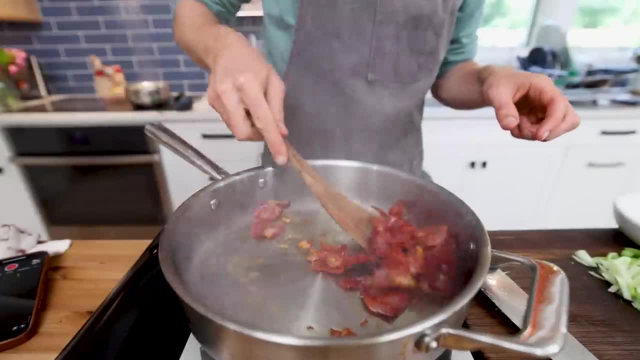 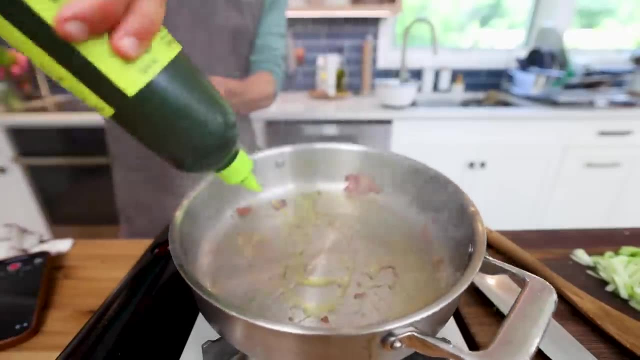 Done, So that is perfect. There's a fine line. You definitely don't want to overcook it, Just nice and rendered and crispy. We'll get that out. Looks like we need just a little bit more fat In with our fennel. 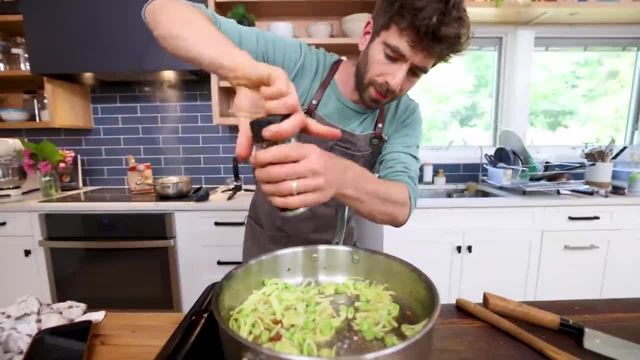 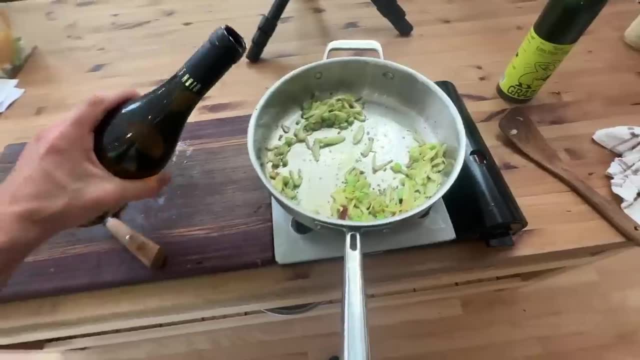 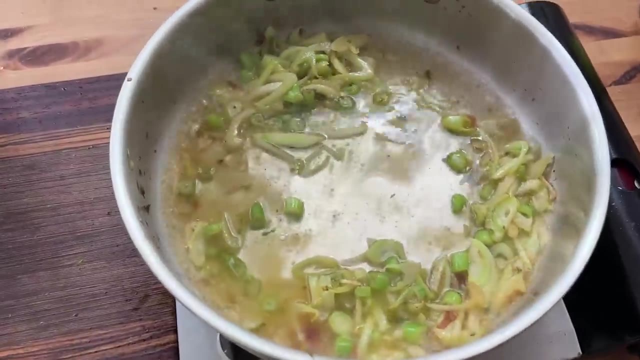 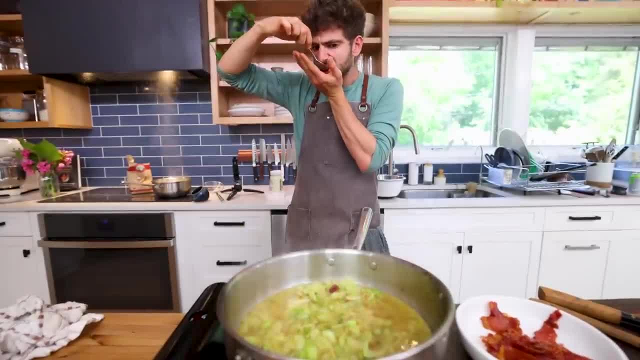 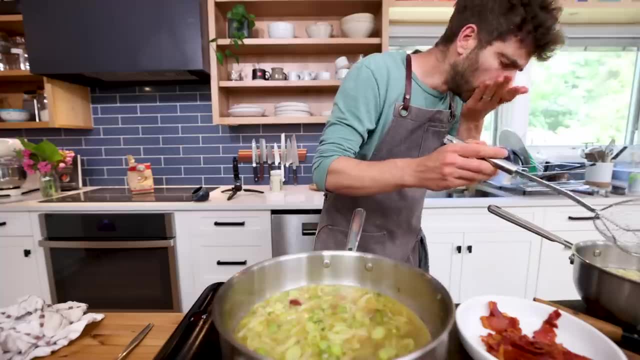 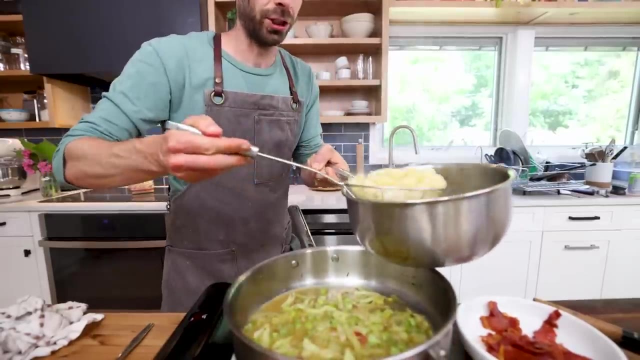 going to give this little sauce a taste. Yum yum, yum. All right, Already reduced pasta, Let's just try one shell to make sure. Perfect Right on time. And this is still liquid. It's not going to be thick, but once we add the starchy pasta, everything's going to come together. I'm thinking. 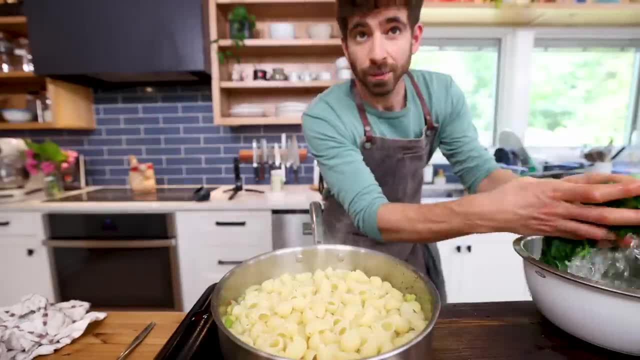 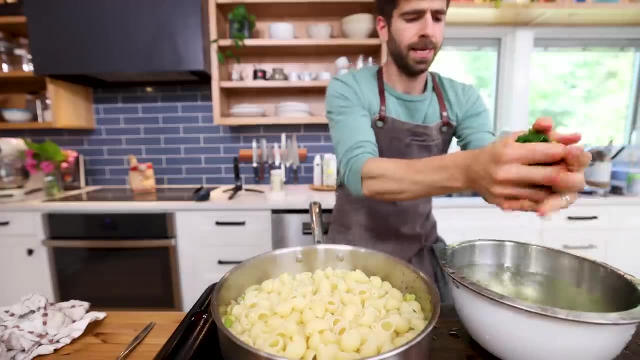 wait a minute. This is feeling a little bit lackluster, And that's because we need to add all of these greens, So I'll just take these and squeeze them into the pot. And then we're going to take these and squeeze them out And they're already cooked, So I'll just give them a quick. 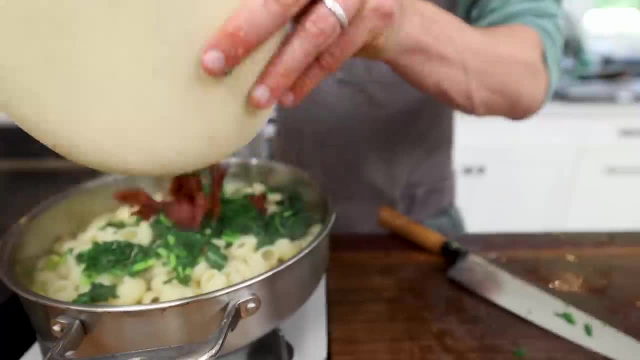 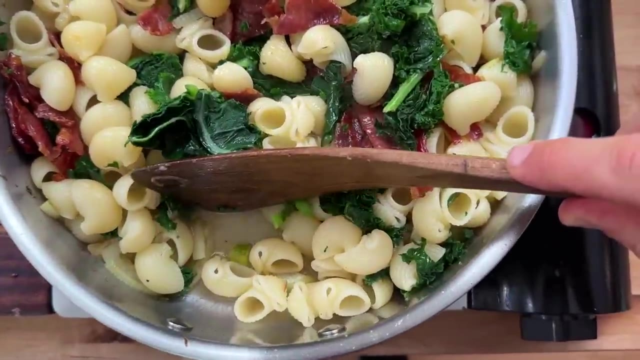 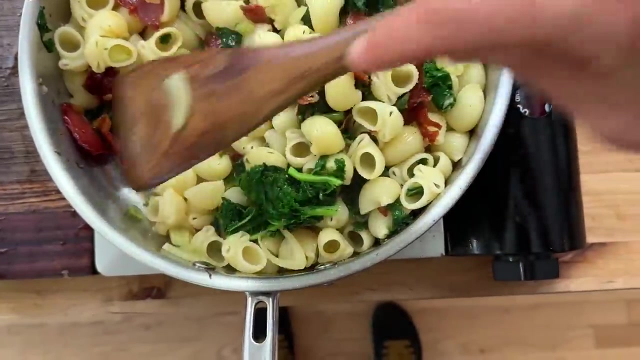 slice-ity, dice-ity. Get that in there. Look how good that looks. Get that in there. Is that really five ingredients? It feels like more, So insane. And now we have one main goal: Take all of this liquid, this wine sauce, and just cook it in with that pasta until it fully absorbs and gets nice. 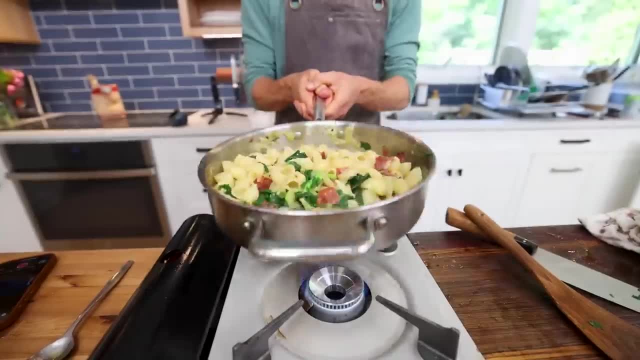 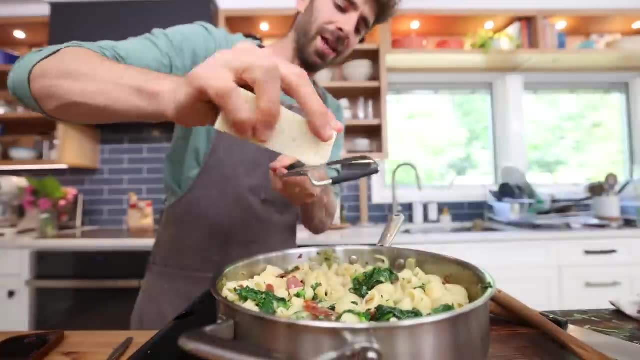 and saucy, which is already happening in a matter of 30 seconds. All right, I'm flying in a major cheat code. This Is some pecorino, which is optional depending on how you look at it. Kind of essential right now. 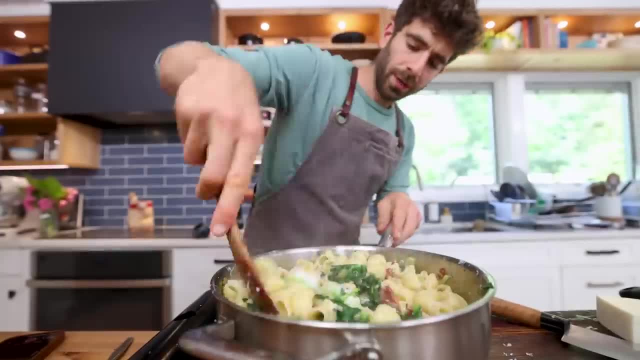 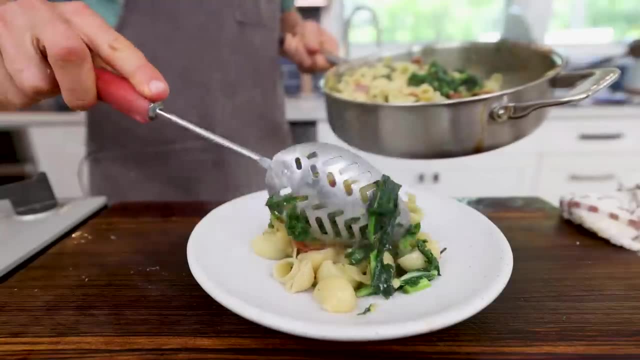 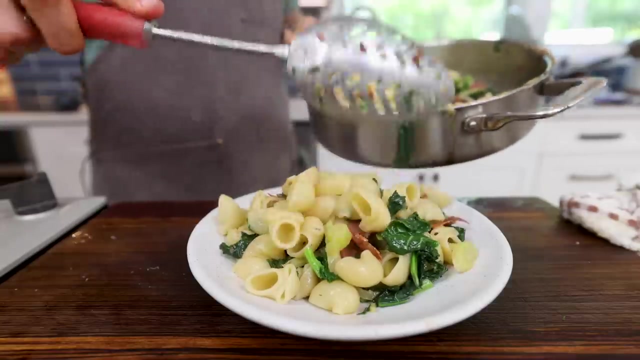 So that's six ingredients. I have failed And we'll just work that in and we'll serve it up. Oh yes, Wow. I guarantee if you go to Italy, at the core of every good pasta is going to be five to seven ingredients. Italian food is simple. It should be simple. 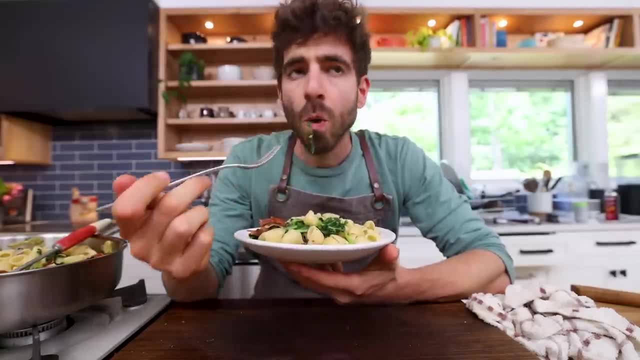 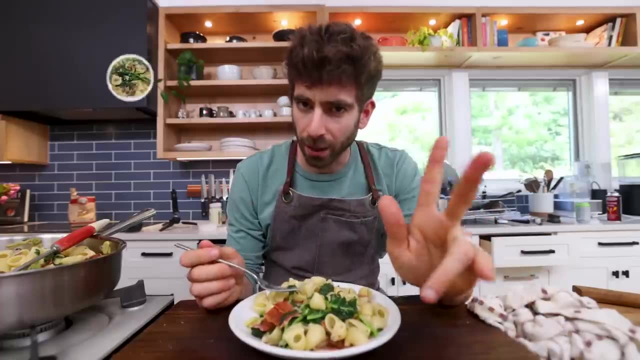 but it's how you craft and care for those ingredients. Mm-hmm, Oh, that's really interesting. This tastes so similar to one of my favorite pastas of all time, which is a broccoli Robin sausage orecchiette. The kale and theắmone are doing a. 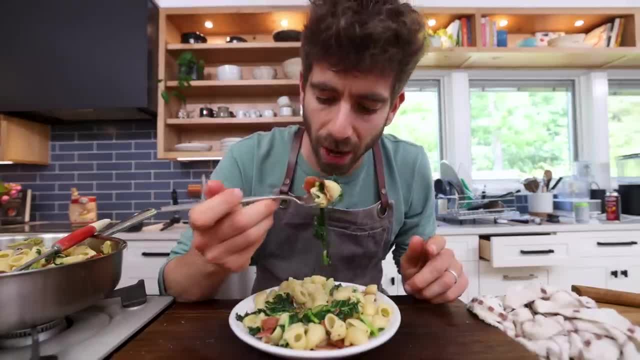 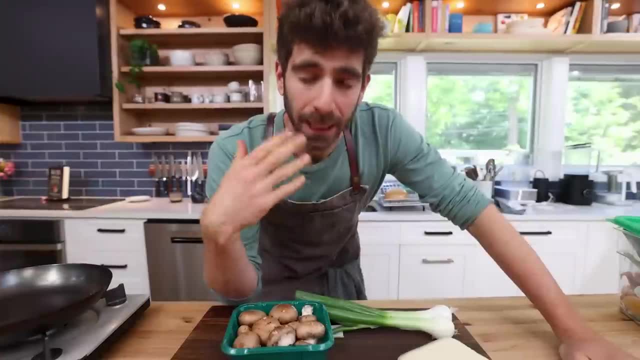 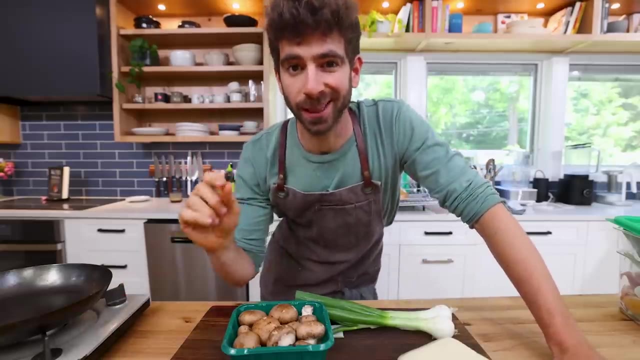 very similar job And I love the combo there. I didn't expect that. That's damn good. So, as you can see, with the last two meals, things can get a little carb-heavy from time to time. I'm eating a lot of rice, I'm eating a lot of pasta And sometimes I'm just a little carved out. 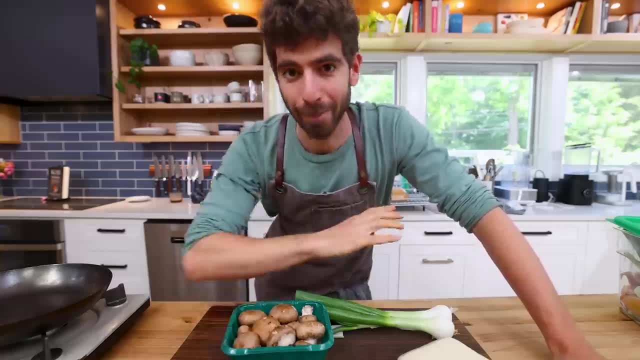 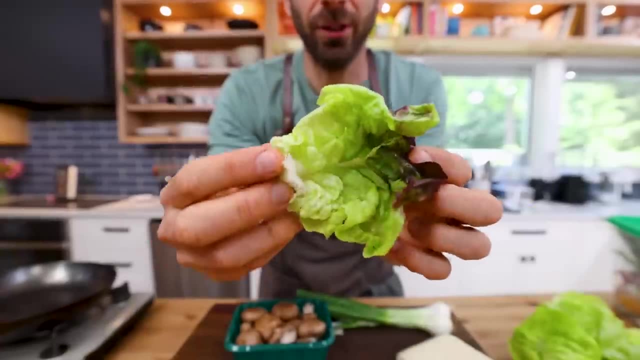 which is when I, Whenever I have meals with a girlfriend, I'm like this is gonna be good. I'm, I am calling on the lettuce wrap And we have this beautiful bibb lettuce. I mean, look at these cups. That right, there is a vessel to hold something. 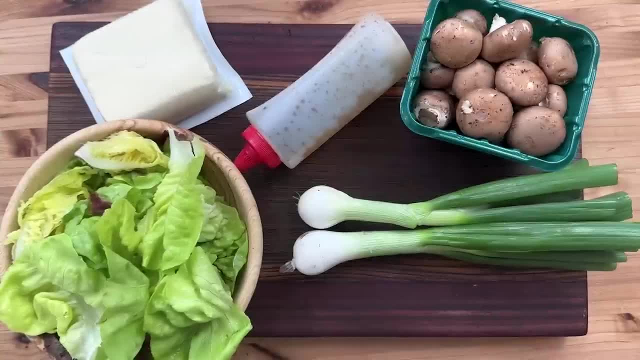 And what I like doing, especially with minimal ingredients, is just making a stir fry and serving it in some lettuce, And that's exactly what we're gonna do. First thing I'll do is just pre-eat my pan on a low heat. 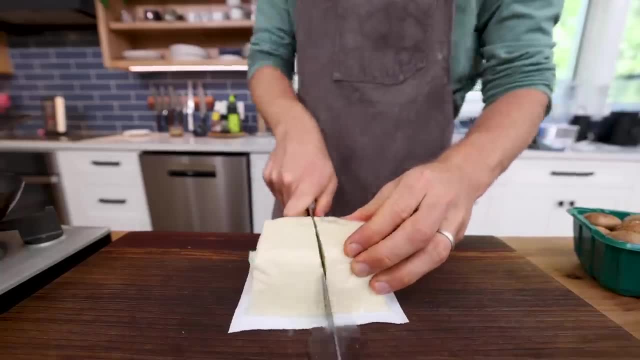 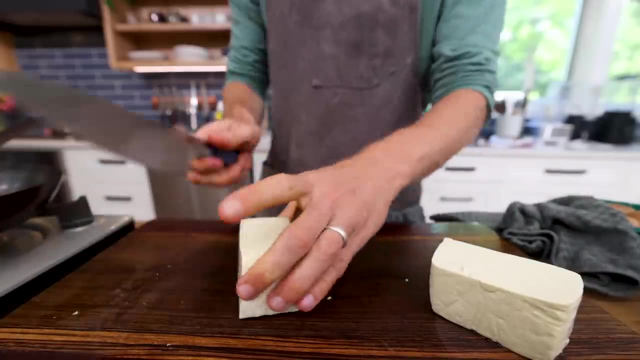 sharpen my knife Now. we've eaten a lot of meat, so I've got a block of tofu here to keep things vegetarian, which is filled with water. Now, to get this crispy, we actually don't have to remove all the water, but just soak up some of that excess water. 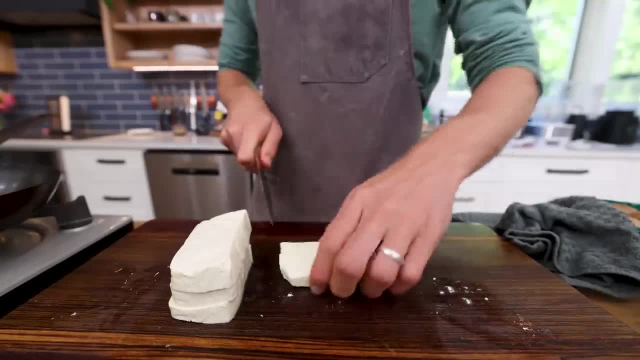 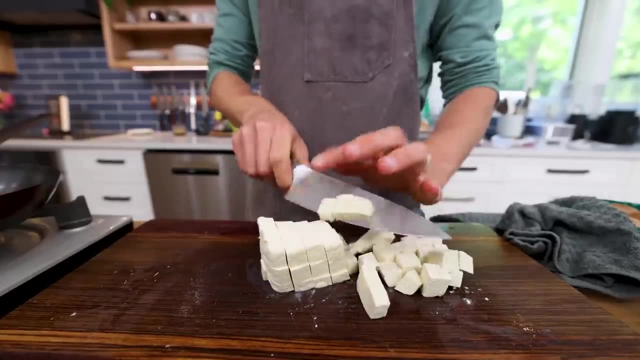 I think this is enough. I'm gonna save this piece And we're just gonna make little tiny cubes, just like that- Same as these here- And then toss that into a bowl. To make it super simple, I'm just gonna spray. 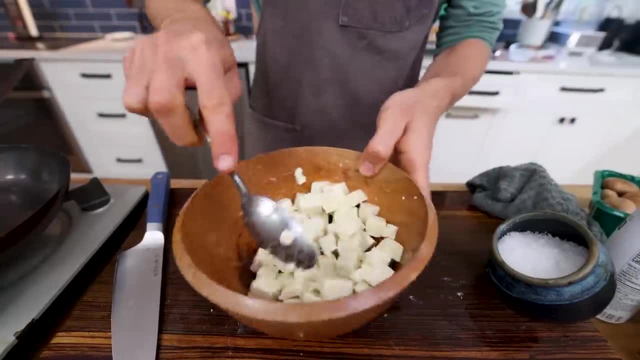 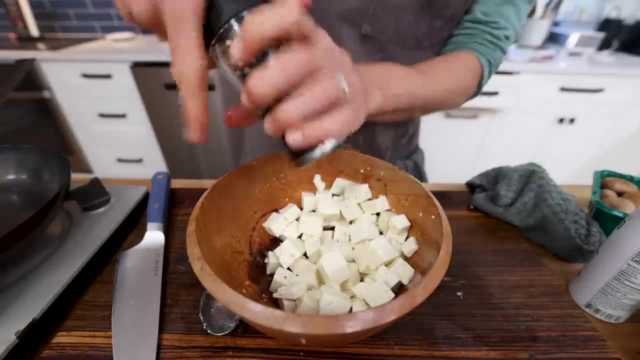 Got some avocado oil, Since we're air frying. the beauty is they can still be a little wet and they don't need that much oil to get crispy. And just a little bit of salt, a little bit of pepper, All right. so these are getting air fried. 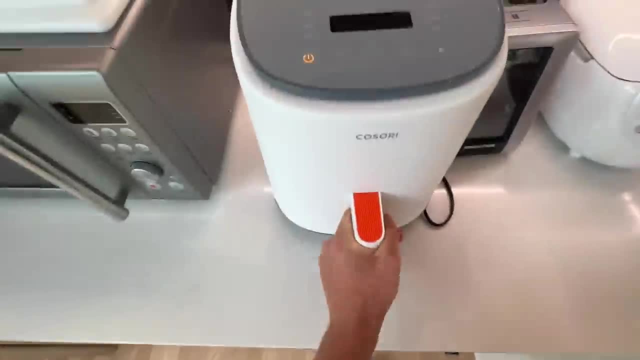 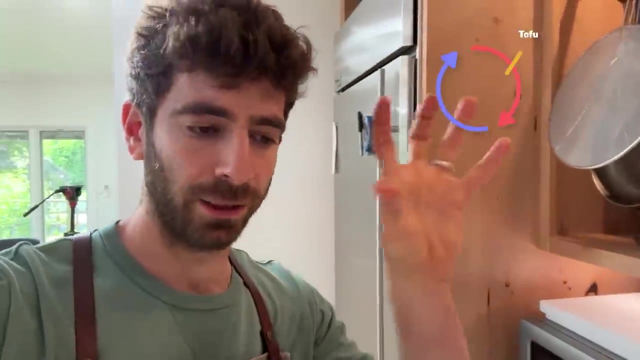 We'll dump those in, spread them out somewhat evenly And we're gonna go high heat- 380.. We'll start at 10 minutes And what's happening here is all this convection heat is gonna simultaneously dry out the tofu a little bit. 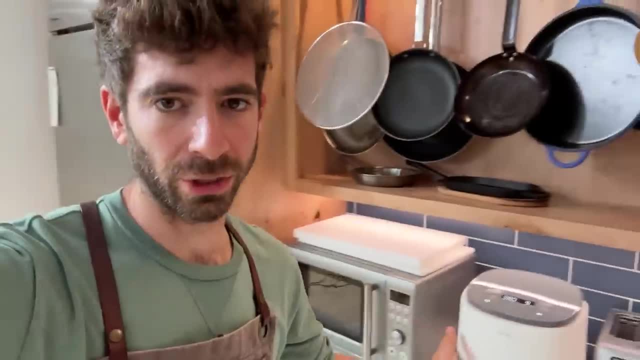 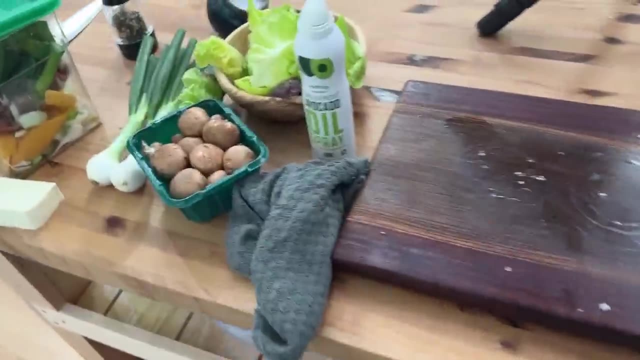 while getting it crispy from that oil coat. And it's just so much easier to cook in an air fryer than deal with flipping it in a pan and all of that nonsense. Game changer, Now we can start chopping up our ingredients to build out this. 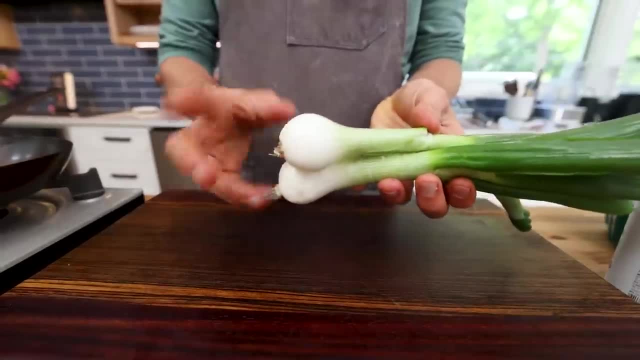 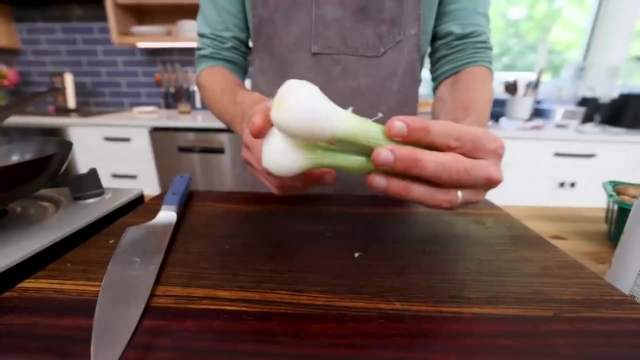 Stir fry. We'll wipe this board down, So here are my spring onions. I'm just gonna use the white part. We'll save this for garnish. When it comes to five ingredients, we take advantage of everything, And this is gonna be the equivalent. 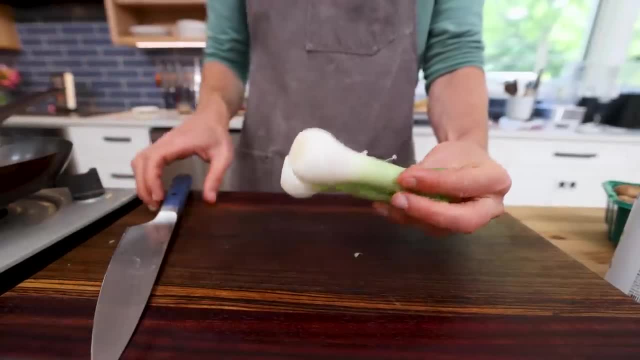 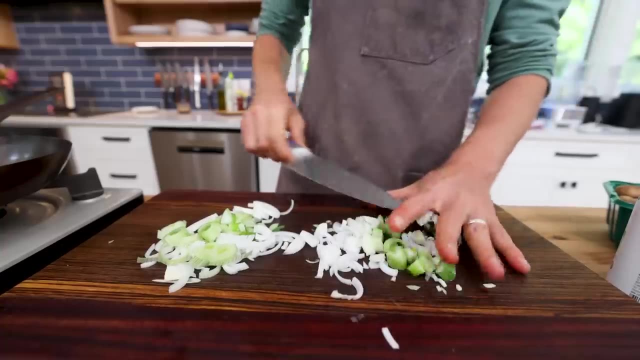 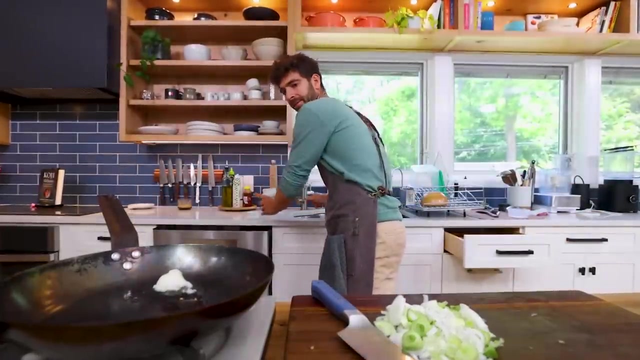 to maybe half a medium onion or one small onion. We'll just slice right through it, Super simple. All right, so our pan is preheated. I'm just gonna add a little bit of fat to the pan. Use whatever oil you have. 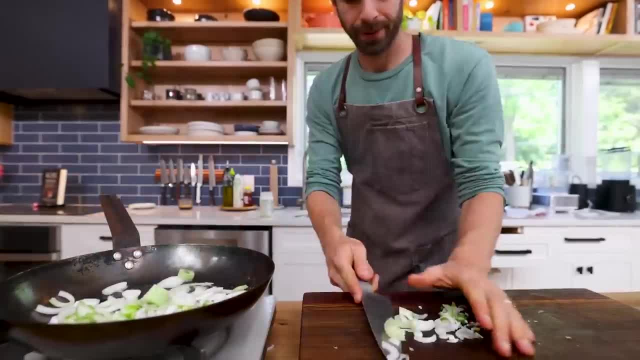 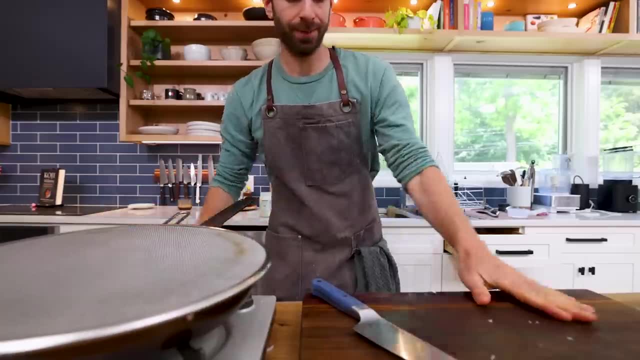 And then I will start Frying up these onions. We're working with some decent heat here, which is when I like to bring in the splatter guard, Keep things clean, And the only other thing I need to prep are these mushrooms right here. 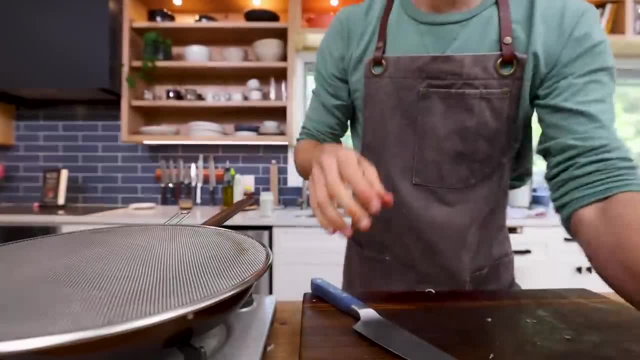 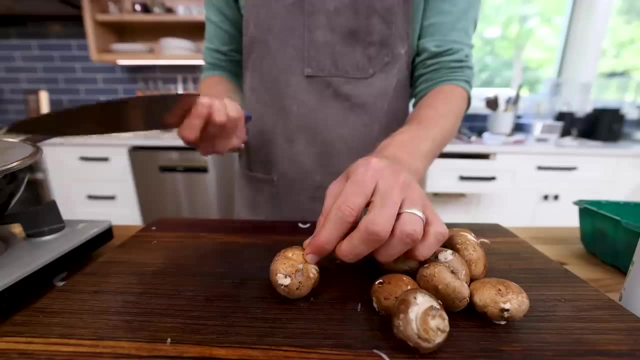 The standard creminis. you could use shiitakes or really anything you can find. These do need a little bit of a clean. it looks like Give them a quick wipe down And for me, the quickest way to cut a button mushroom like this. 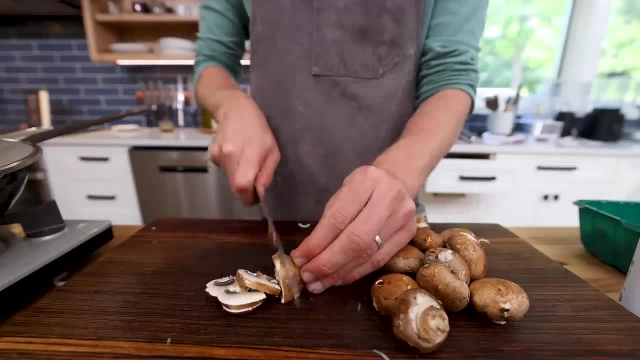 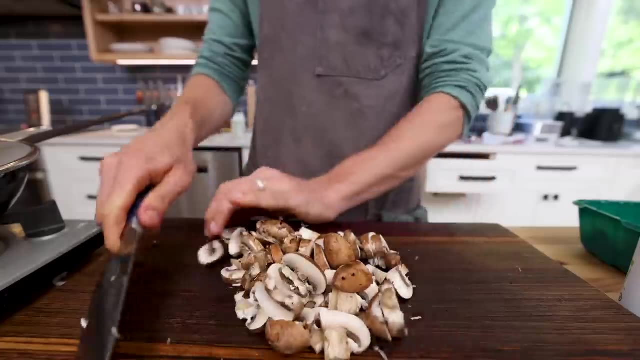 slice off just the little end piece. place it flat Rattle through Slice. place it flat rattle through Now, once we have some decent color here. onions are a little soft on with the mushrooms And don't be nervous if your mushrooms absorb up. 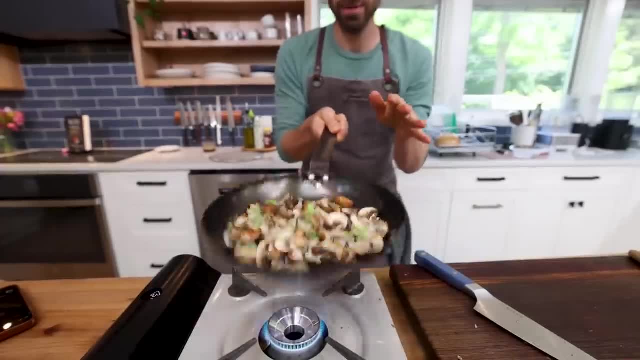 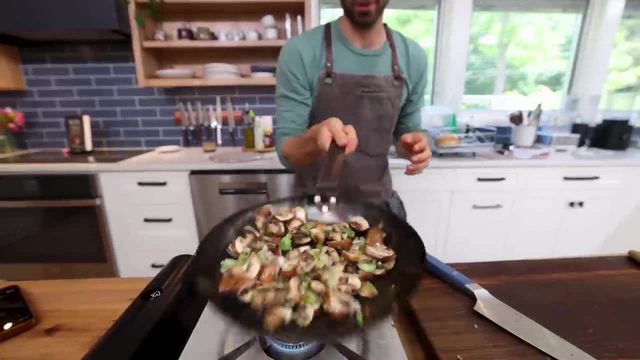 any excess oil. They first suck up all of that moisture. You can see the pan is pretty dry here. Then they start releasing that moisture back into the pan, which makes it a little bit easier to stir fry. So don't get nervous and just start dumping in a ton of oil. 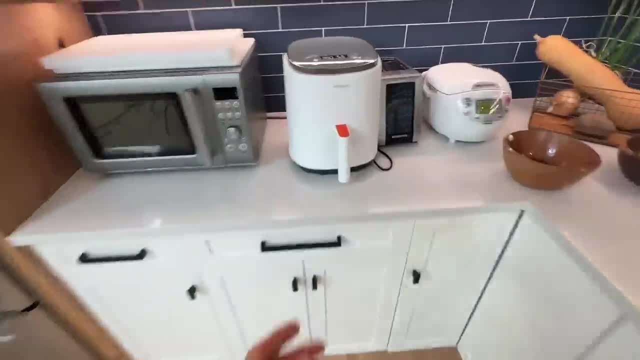 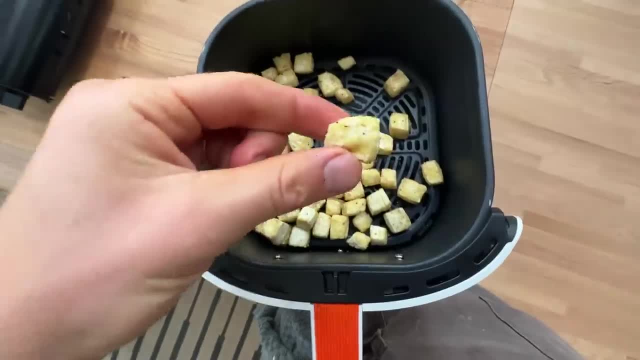 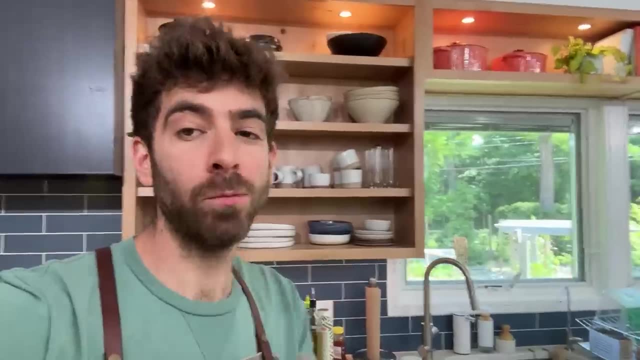 Check out our tofu. Oh yeah, See you just give it a shake So you can see they still have some nice moisture in there, but they're getting crispy. Not recommended to try one this hot. I'm a trained home cooking professional. 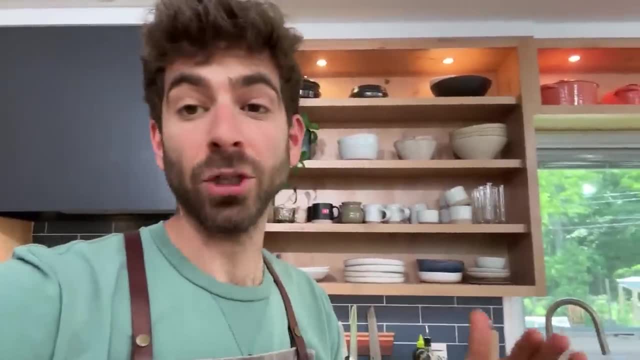 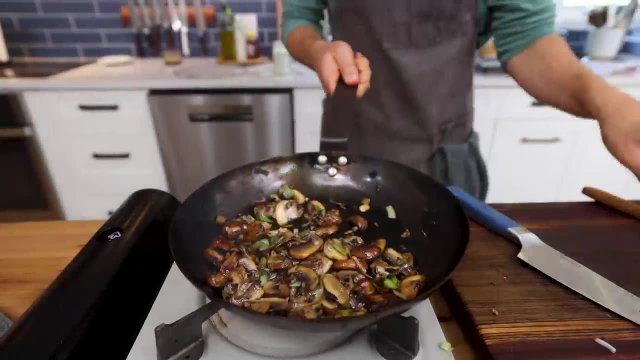 Mm. tastes like authentic fried tofu that you'd get from Chinatown. So good. I am gonna give it three more minutes and it'll be perfect. So you can see, these mushrooms have browned up really nice And actually they haven't released that much moisture at all. 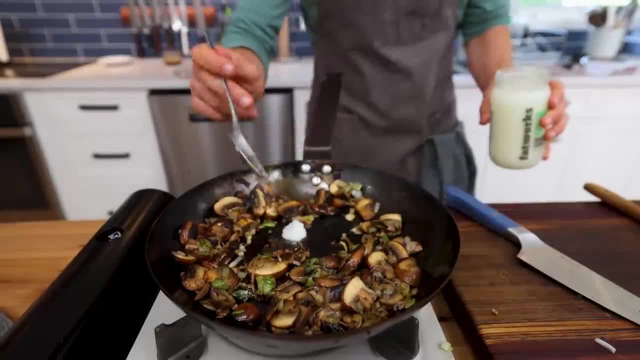 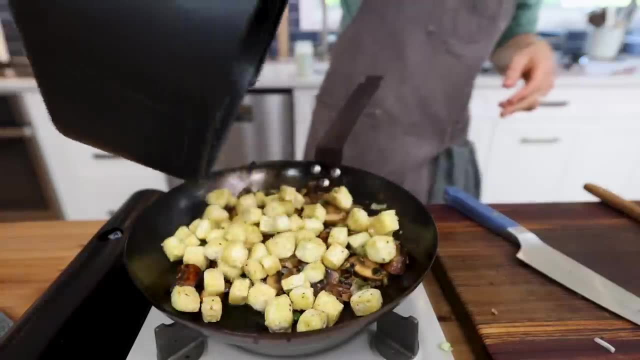 And now that they've broken down, I feel comfortable adding just a little bit more fat, Tiny bit of salt, And here we go. I'm going right in with the crispy tofu. Now we've got our stir fry, but we need a little extra flavor. 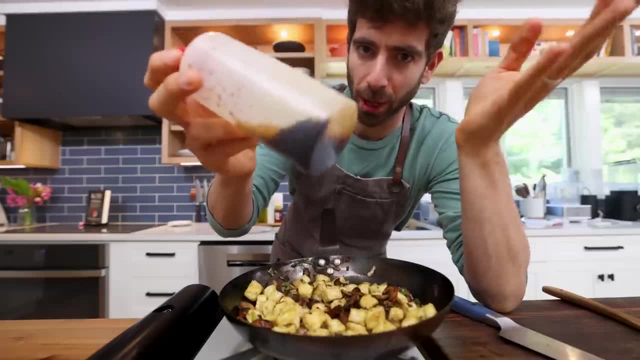 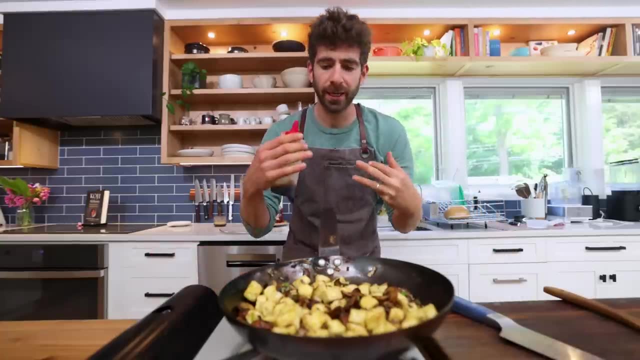 And here's my cheat code. This is just some store-bought Asian style barbecue sauce. You can use a teriyaki sauce. You can use an American style barbecue sauce, Just anything. you want to add a little bit of glaziness, to add some of that sweet salty kick.